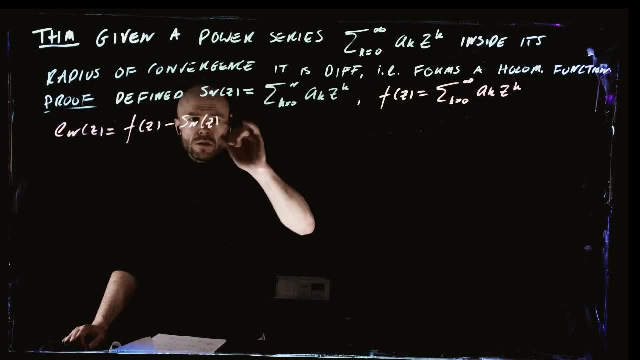 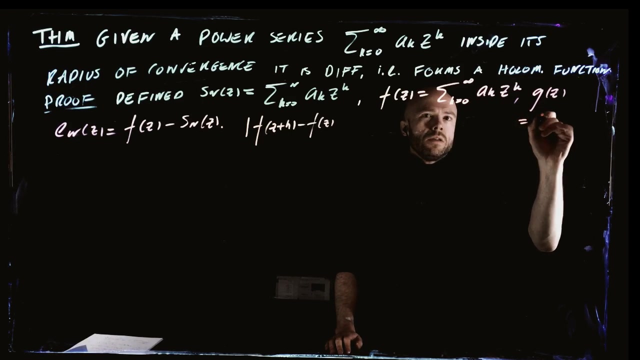 Okay, Like this, And I think that's all that we defined Right, And then we were considering right this thing. so we were considering f of z plus h minus f of z. we also define g to be the derivative. so g of z is the sum from k equals one infinity, k a to the k. 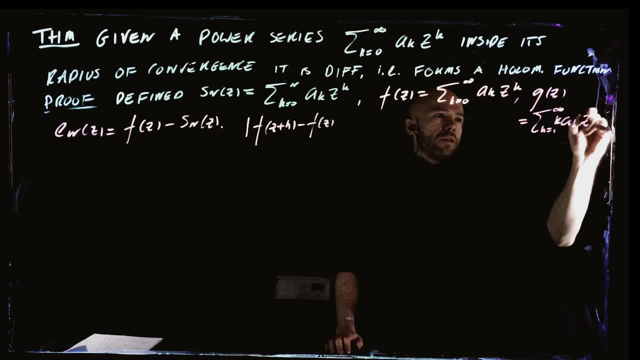 z, k minus one. so we define this thing like this, right, and we broke this up into various little pieces using these various devices. the first thing we did was to write this quotient in terms of e, n and s, n, and then we wanted to. well, i'll just write it. 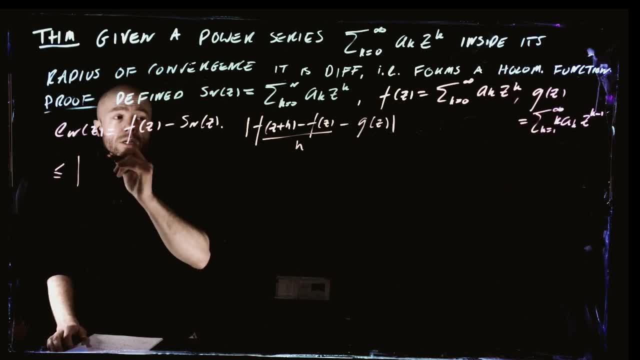 it's easier to write it than to say all these words. so What did we do? We wrote S n z plus h, minus S n z over h, And then the actual derivative, And it's not hard to show that this thing will be small. 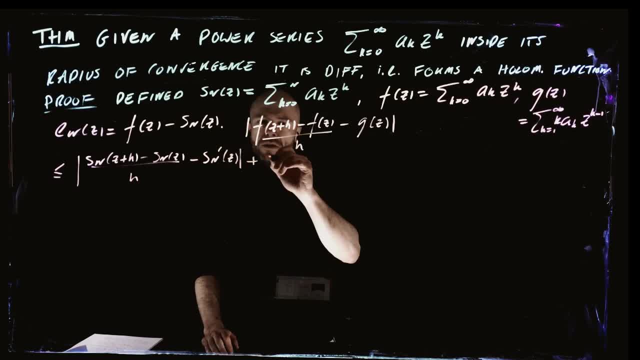 because this is just a polynomial, it's differentiable. And then we had S n prime of z minus g of z. Again, this is obviously controllable. And then we had this thing: E n of z plus h minus E n of z over h. 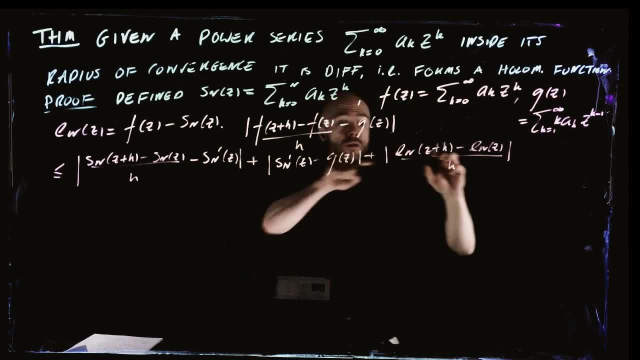 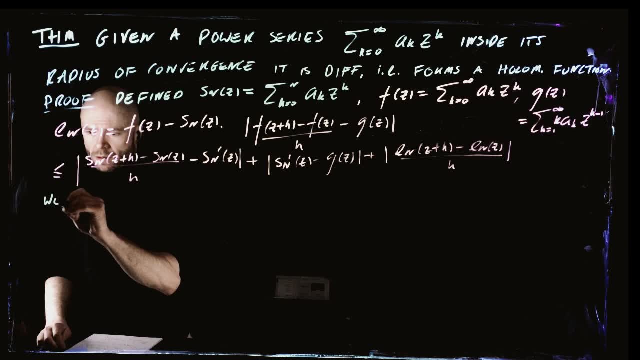 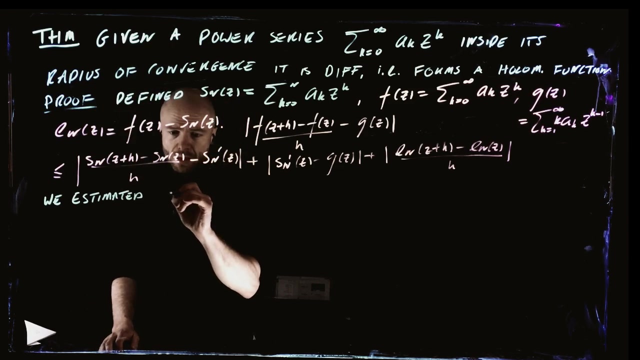 Yeah, And we got to the point of estimating, or trying to estimate this thing, And we estimated The following: So we estimated that this thing, k minus z to the k over h itself, this thing absolute value was less than. 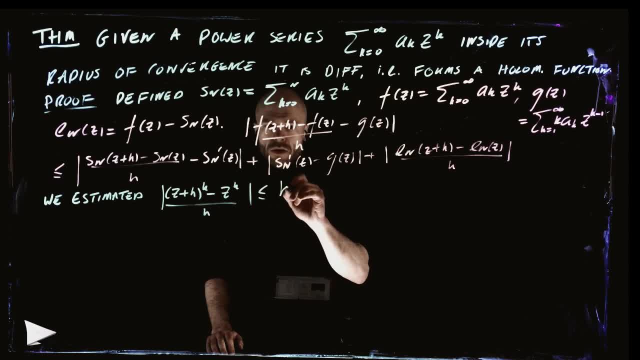 k, r to the k minus one, where r is the radius of convergence. So this is where we were, This is where we were. Okay, we're going to use this to estimate this guy right here. So notice this, that this guy. absolute value of E, n, z plus h. 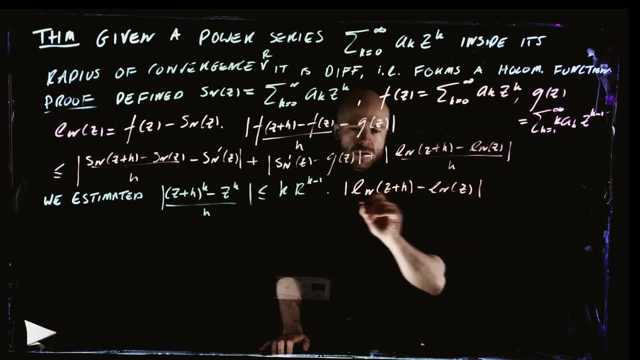 minus E, n of z over h, This is going to be less than and equal to the sum. So we're summing from: k equals n plus one to infinity. Now maybe unmute yourselves, because I'm not going to be able to hear very much anyway. 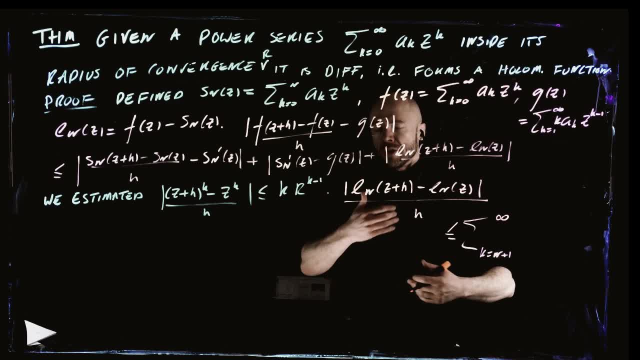 And all I'm hearing is weird, static. So sorry, sorry again. Now mute yourselves and then unmute. if you want to try, Wait a minute, Just win the lottery and speak to me and see if it goes through. So mute yourself and just unmute when necessary. 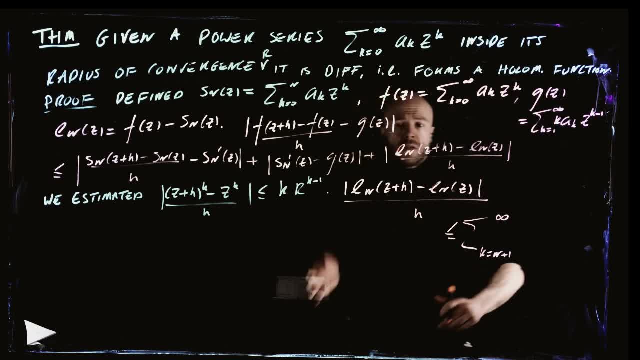 All right. so this thing, you know, just using the definition, is going to be less than the absolute value of all of these coefficients, right, E, k, you know, and then z plus h to the k, minus z to the k. 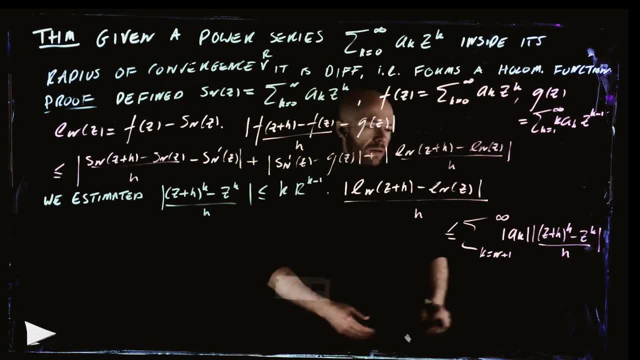 Say that. so this is the thing which we have to estimate, right. But we know that this is less than the sum. k equals n plus one to infinity, not a k. And then this thing we've just estimated like this: k after the k minus one. 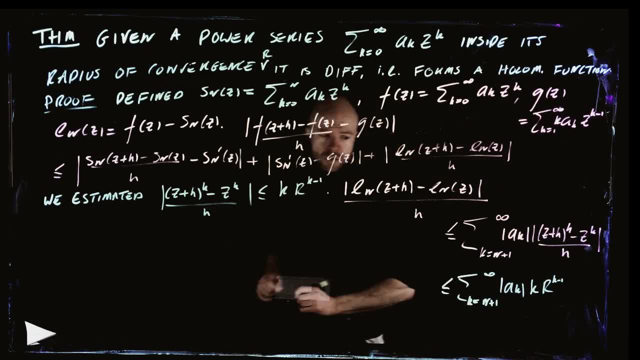 Yep, like this cool. But this thing we saw from the previous proof is the tail end of convergence series. right? This is the tail end of a convergence series because this r is the r we get from this Halimard. represent this Halimard formula, right? 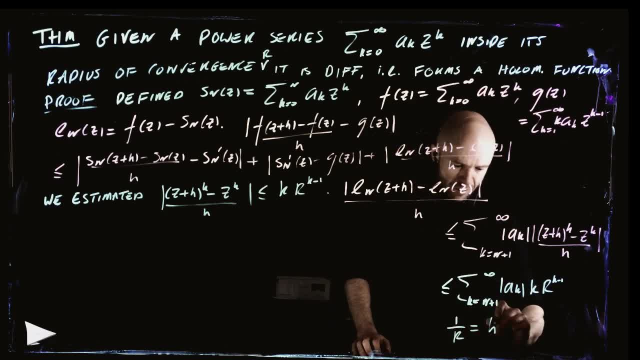 So we call it one over r was the Lim soup, as k goes to infinity of the absolute value of a k. one over k. you know This r looks a bit like a k And that was strong enough to mean that these terms. 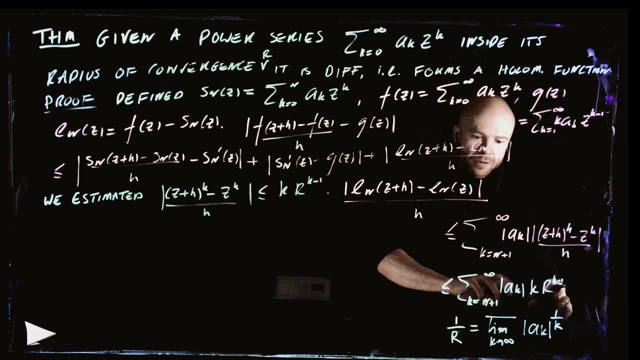 right here will be bounded by a geometric series and therefore they converge right. So we are fine to show that this thing here gets as small as we like, so long as we pick n to be as large as we like, And it's independent of our choice of h. 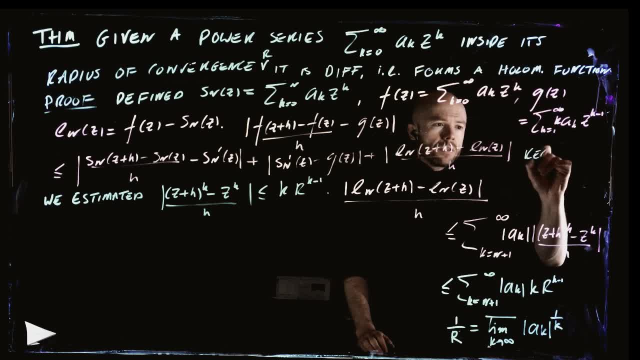 because all we needed was that both z and z plus h belongs to the ball of radius zero, rate of r around zero. in other words, they're inside the radius of convergence. That's all that's needed for this estimate here that we talked about last time. 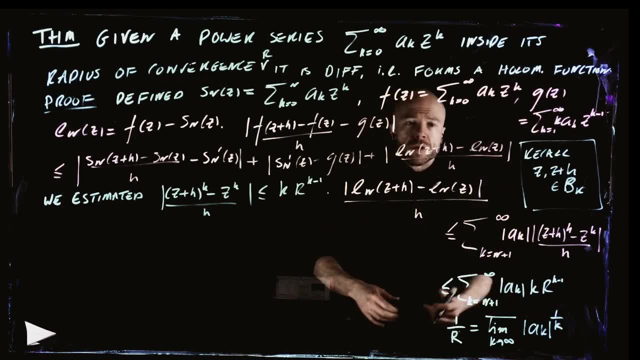 So this part right here we can actually control. we can actually get something out of. We can more than that. we can make it as small as we like by taking n to be sufficiently large, and it's independent again of h. we just need h to be here. 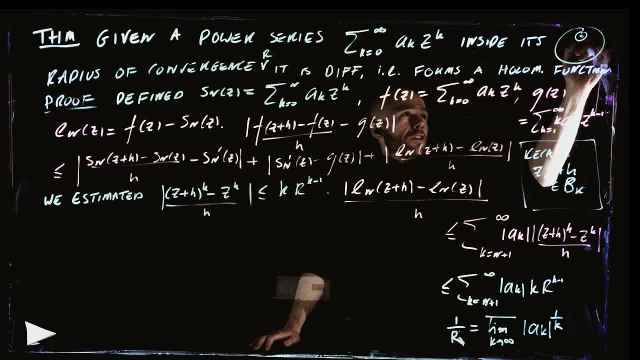 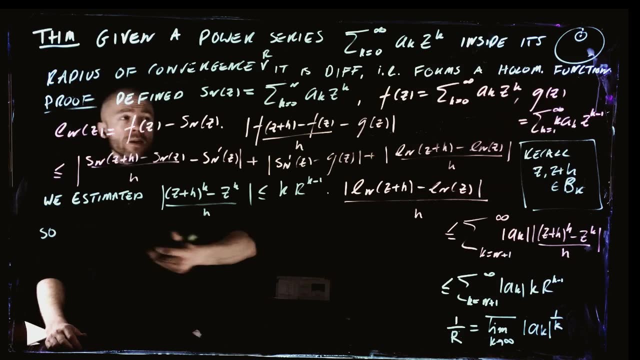 So z is somewhere inside our ball. we just need h to still be inside our ball, so there's some fixed radius where we can get any small h and this will be true. yeah, So in particular, remember we took an epsilon right at the beginning, or at least you know. 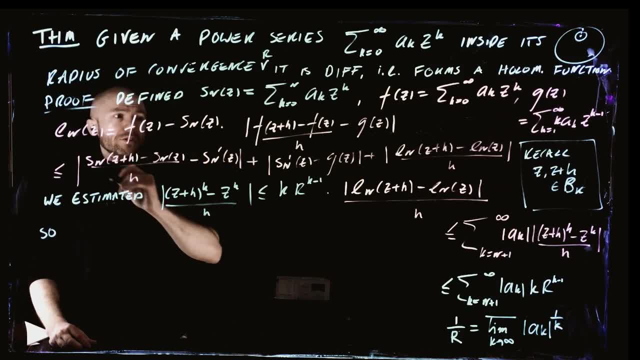 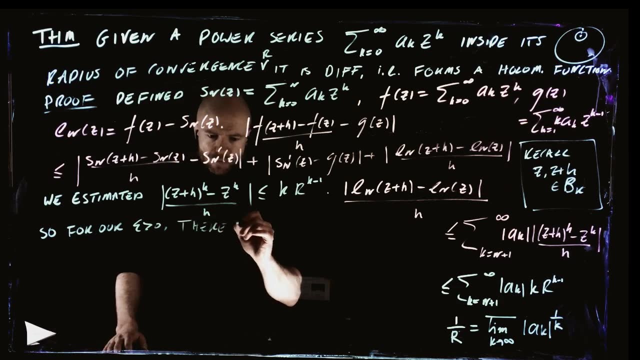 the previous proof, So I should say it here. So for a pre-chosen epsilon, there exists some capital N zero, such that this guy right here E capital N zero. well, let's write it more generally, but we don't really need to. 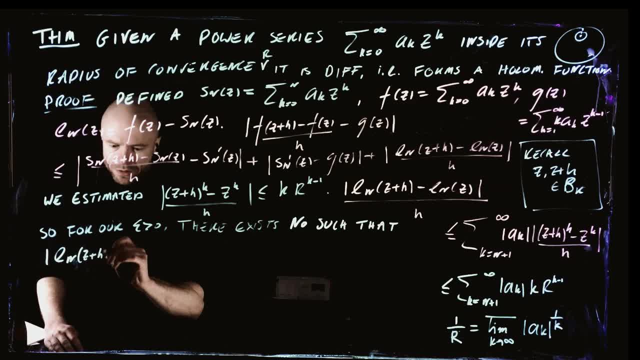 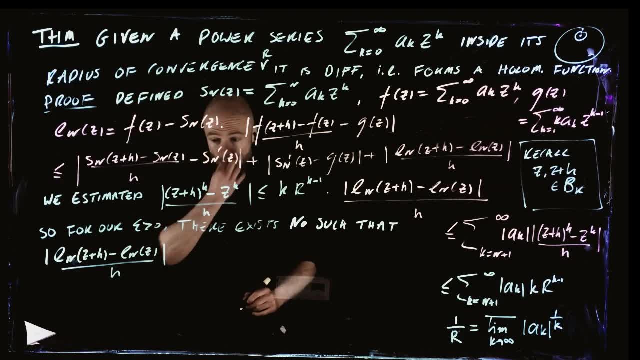 But let's write it more generally: E of z plus h minus en of z over h. This thing right here, L is less than or equal to epsilon for all n big or equal to n0, just from this estimate. So this guy, this term here that we had to be concerned about this guy, is under control. 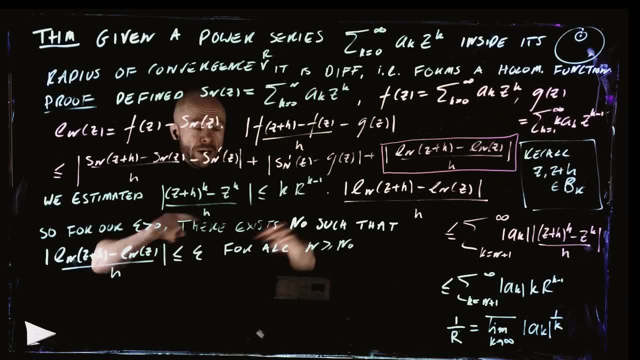 now. So we're just going to work with our n0 from this point onwards, because that's going to be good enough for us. So we're going to use this estimate here and we're going to take n0 inside all of this. This will be less than epsilon again for all h, such that z plus h is inside the radius. 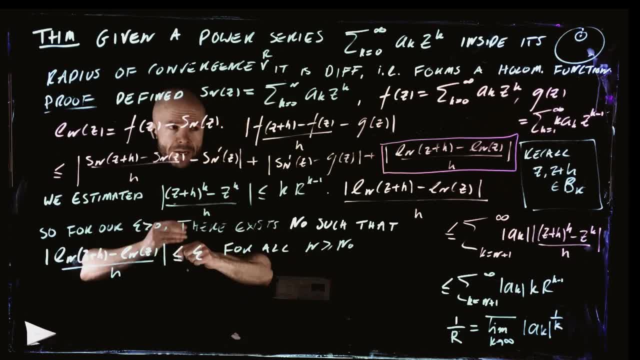 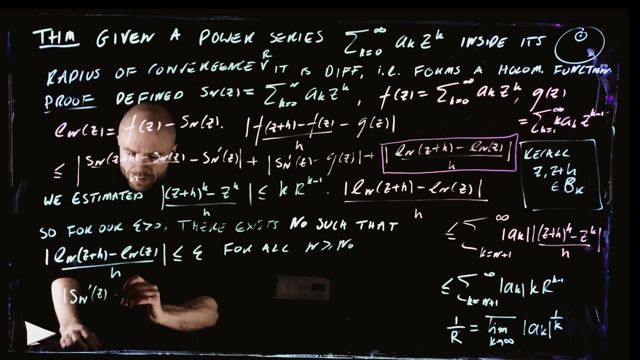 of convergence. So now we have to think about the other two terms And we have this thing to control and this thing to control. Let's control this thing first of all. Well, what about this guy? Sn prime of z minus g of z? Sn prime is just this polynomial given by the first n terms. 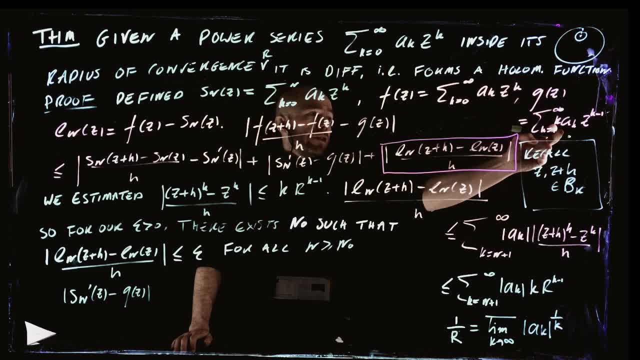 So if we differentiate it- and g of z is what we get from differentiating term by term- if we take the difference, then we're just going to have the sum from n plus 1 onwards, So this thing is actually just equal to the absolute value of the sum from k equals n. 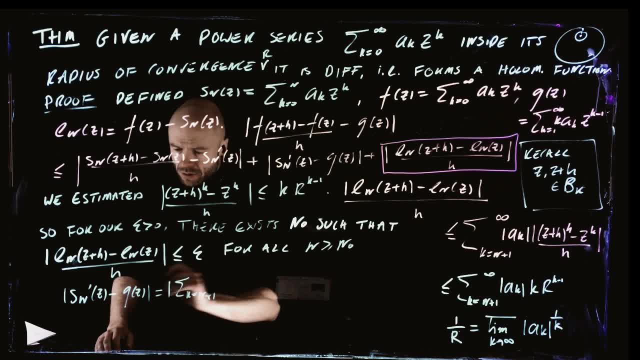 plus 1 onwards. Actually, let me do it again. So this thing is just equal to the absolute value of the sum from k equals n plus 1 onwards. So this is n plus n minus 1.. Let's take that and we're going to do n0, because I said I'm going to take n0, of ak. 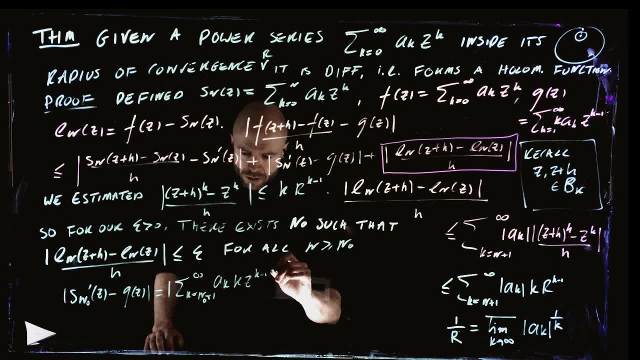 z to the k minus 1, right. And then the same estimate plays out. here: We've chosen n0, such that this stuff is less than epsilon. so this is also less than epsilon. Yeah Cool, So we've controlled two of our terms. 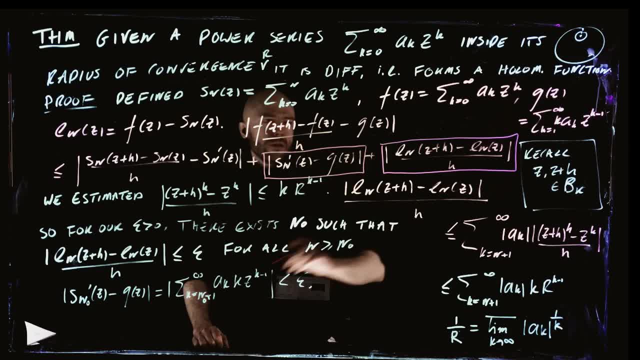 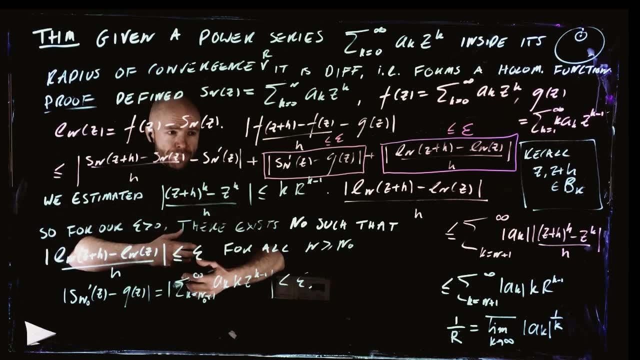 Thank you. So this thing is less than epsilon. this thing is less than epsilon, and our final thing to control is this thing, And again, we've chosen n0, n0 is chosen, it's fixed, and now we have the right to move. 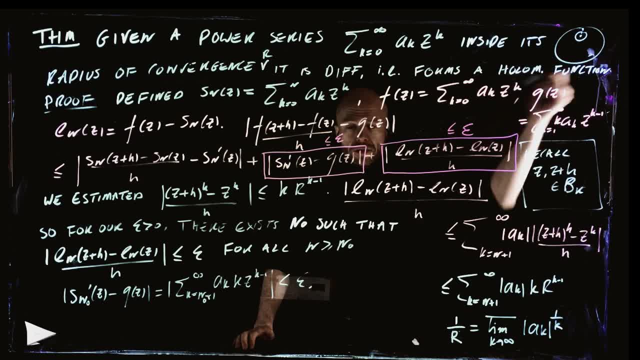 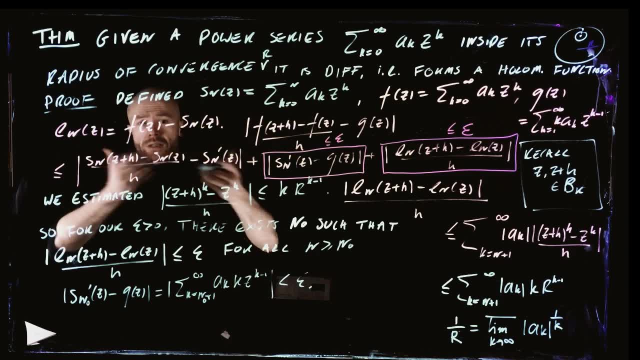 h, because h the only restriction is that it still remains inside the radius r. all of convergence, And this thing right here is just for our fixed n0, is just a nice polynomial, right. So this is just the difference quotient. this is the derivative of the polynomial and of. 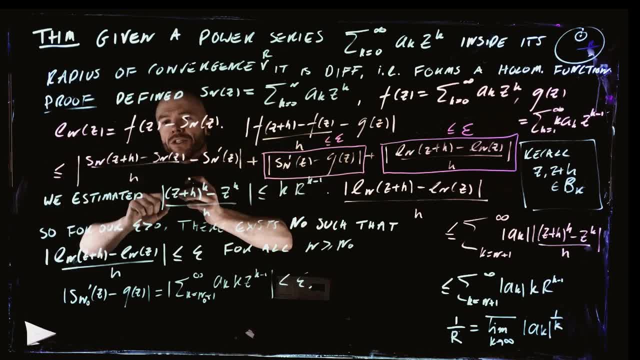 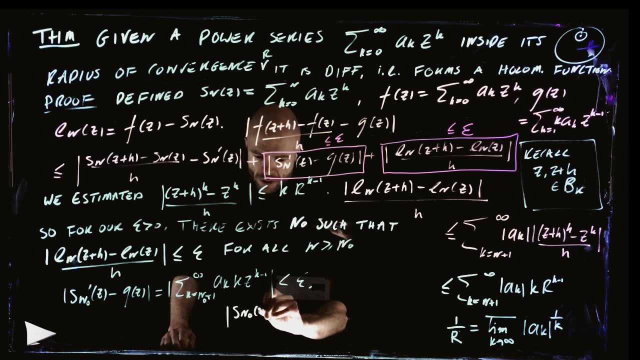 course this thing gets to be as small as we like, as we let h go down to 0 for our fixed choice of n0.. So this thing, let me rewrite it here, this thing s n0, z plus h, n0, n0,, n0,, n0, n0,. 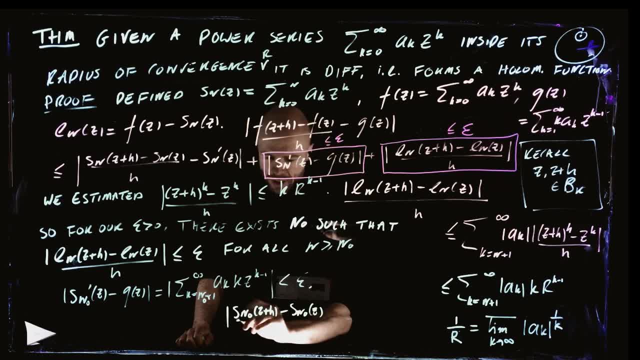 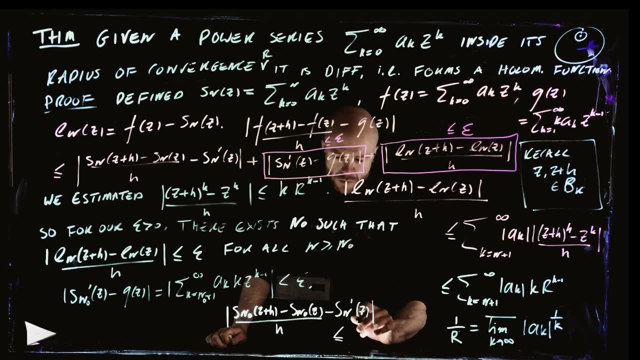 minus s n0 of z over h. okay, minus s n prime of z. This thing is also less than epsilon. for all, running out of space here, let me put this up here for all: epsilon, Okay, Okay. 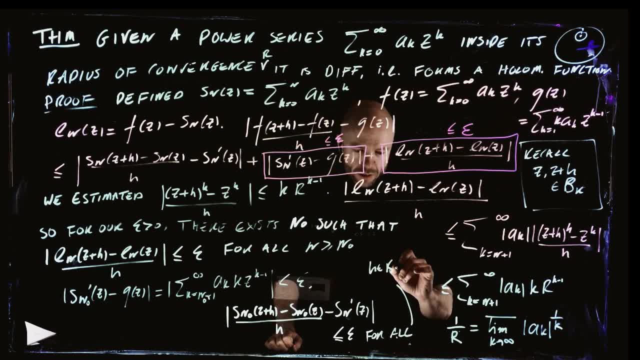 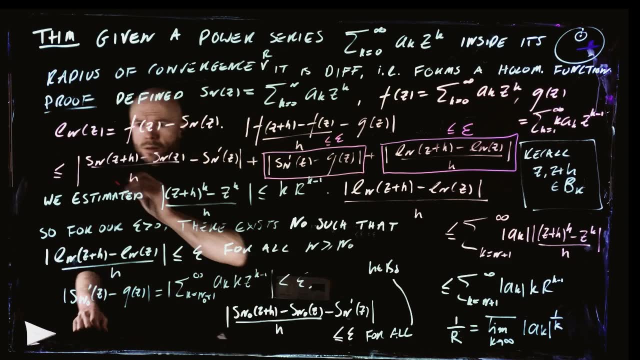 So this is h belonging to some particular radius around 0, just by definition of differentiability. yeah, Cool. So what that means is that this guy right here is also less than epsilon. yeah, So putting these things together, we have that this thing is going to be less than 3,. 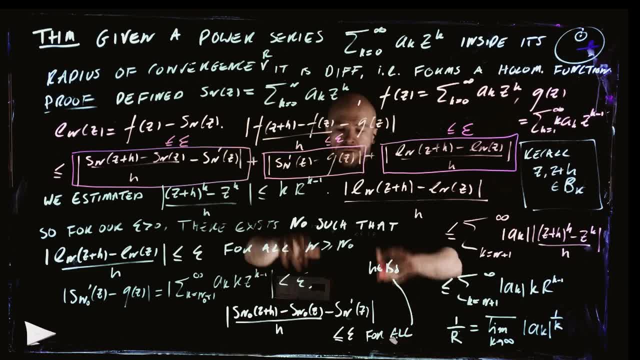 is going to be less than 3 epsilon, right for all h, such that- this is true, which I can just rewrite- epsilon this way for all h comes to a value less than delta, yeah, Yeah. So what's that saying? 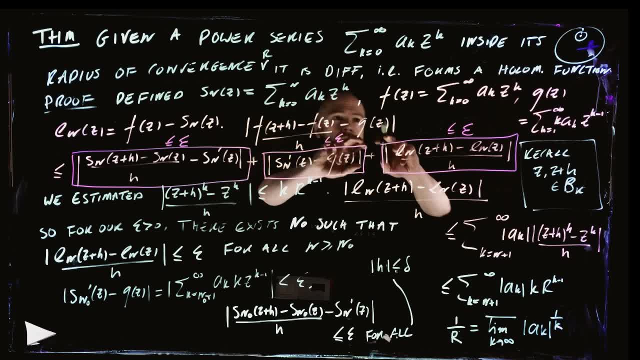 That's saying that this quotient gets as close as we like to this holomorphic function, which you already know is a holomorphic function. We just know that. We've already discussed this already, you know. And so as we take the limit, as h goes to 0, then it is actually equal to this thing which: 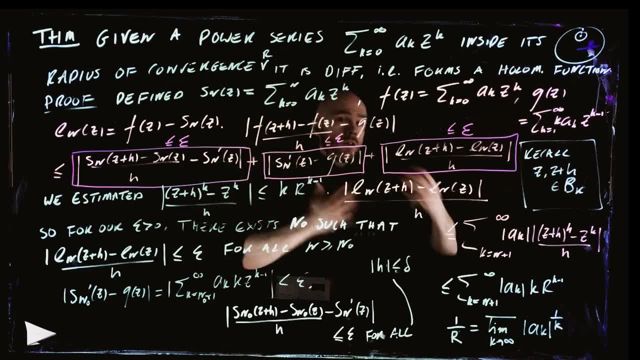 means, firstly, that this limit exists. therefore, f is a holomorphic function, it is differentiable inside its radius of convergence and its derivative is given by this. okay, So we have what I claimed in this theorem, and this powerful thing is saying that inside. 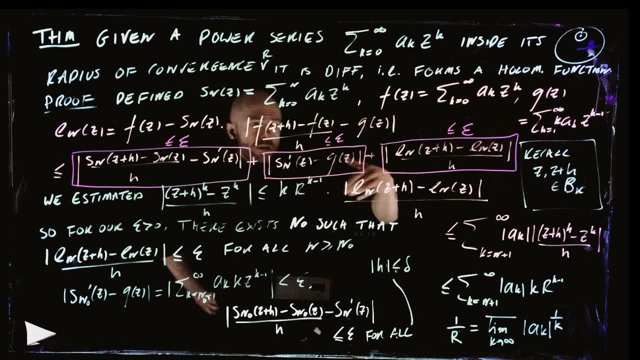 the radius of convergence. we have this In the radius of convergence. power series behave just as nicely in terms of differentiation as polynomials. This expression here for the derivative is exactly what we'd get if we differentiated term by term, if we had a polynomial. yeah, 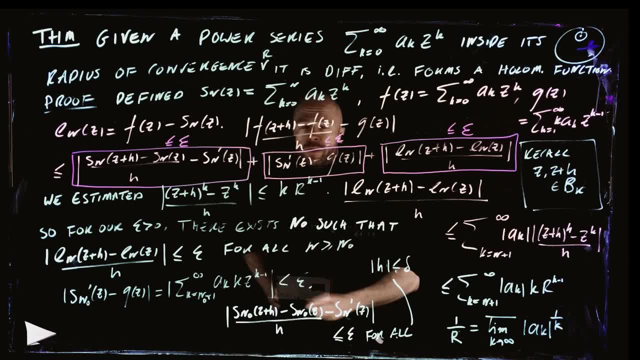 So we have a very nice, strong, powerful result. you know We can simply differentiate any function we can represent as a power series, just term by term. Differentiation is way easier than finding the antiderivative. Nevertheless, there can be some tricky functions to differentiate there. you know some difficult. 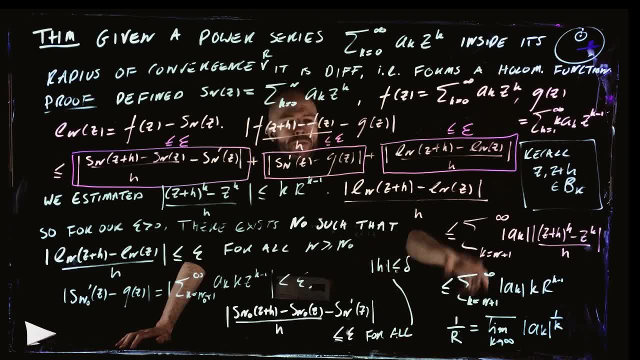 expressions with the quotient rule. whatever mix things up, have calculus students using quotient rule to chain rule in combination. If you have a power series, then differentiation is just a triviality. a triviality, right, Cool, All right. So this says this. 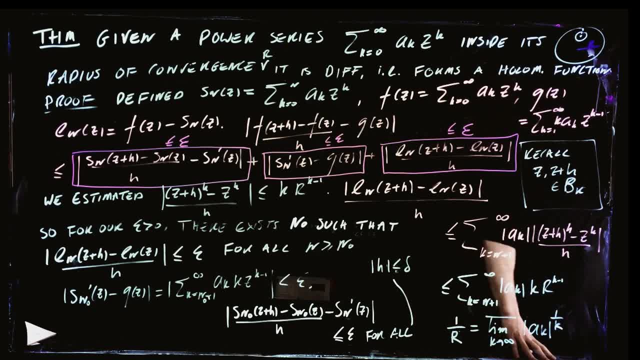 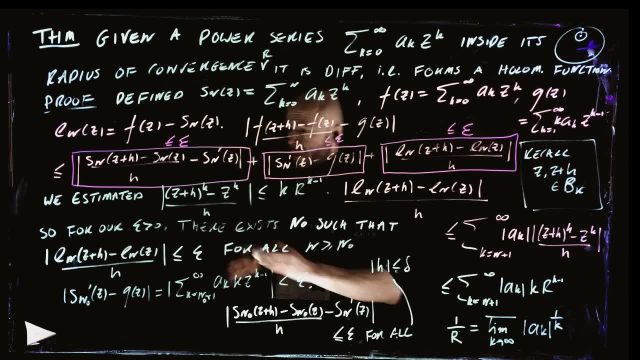 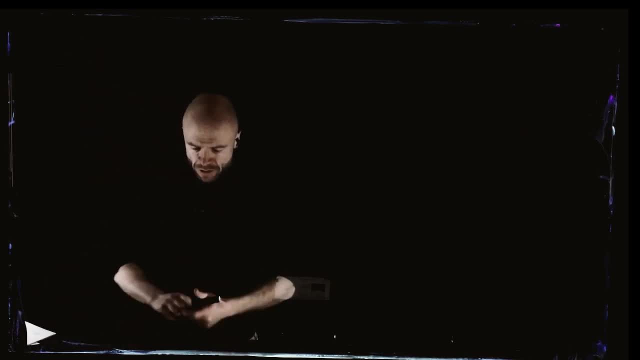 And the other cool thing it says is that we now have an even wider class of holomorphic functions. So we not only have the following function, the exponential function, or the complex exponential function. So if we consider this series, sum from k equals zero to infinity. 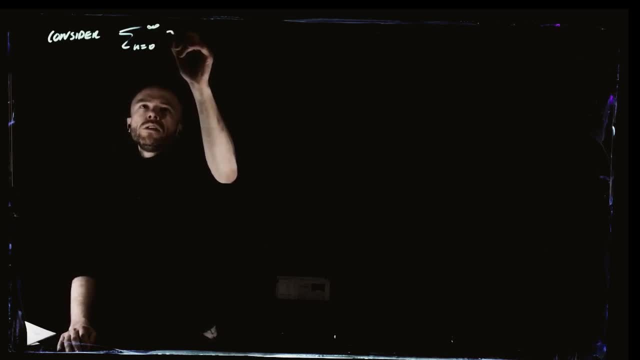 All right, So we have this, So we have this And in terms of infinity, that's the k over k factorial. let's see what its radius of convergence is. So these coefficients are given by this thing. So if we try and take the kth root power of 1 over k factorial, then the lim-soup of this 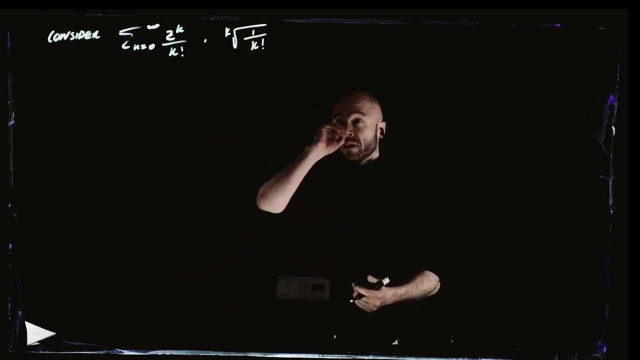 thing is 1 over r. yeah, Lim-soup of this thing is 1 over r. Yeah, All right. So let's estimate this from above. So this is the same as one over the kth root of k, factorial, and we'd expect this to go to zero, as k tends to infinity. 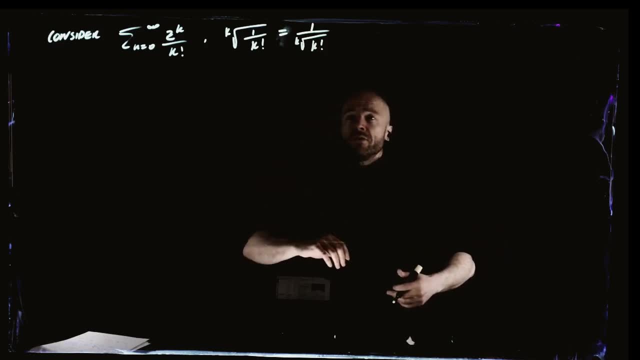 which would imply that the radius of convergence is infinity. So we're gonna be bounding this from above and we know that k factorial is k, k minus one, blah, blah, blah. So in particular it is bigger than what happens when we multiply k over two times k over two. 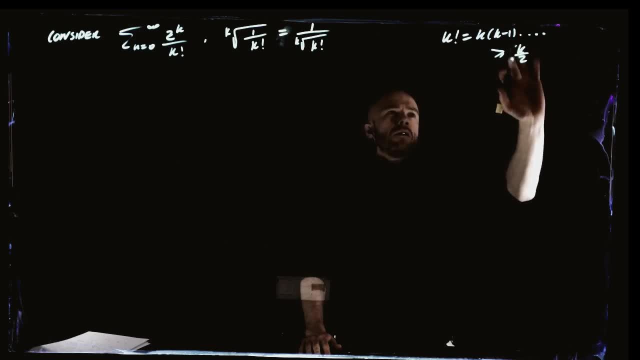 No, no, no, That's not what I want. Bigger than k over two times itself. k over two times right, Because k over two of these terms are at least bigger than k over two. So it's bigger than this, right. 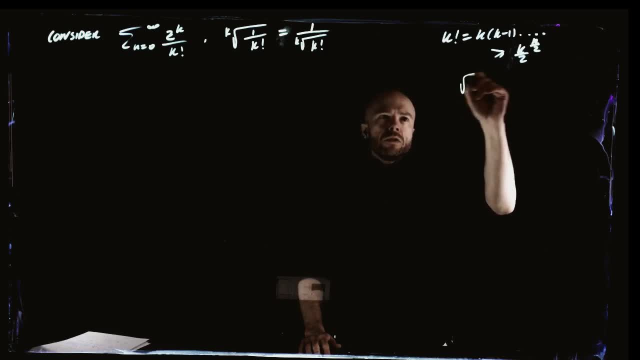 So if we take the kth root of k, factorial, then it is gonna be bigger than the kth root of this thing, which is gonna be bigger than k over two to one over two, which is square root of k over root two. right. 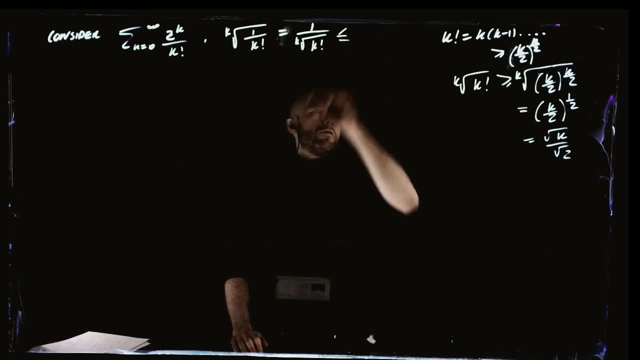 Which means that this thing will be less than root two of root k. Okay, because this thing is bigger than this thing. Yeah, so one over this thing is less than this thing And this thing goes to zero as k tends to infinity. 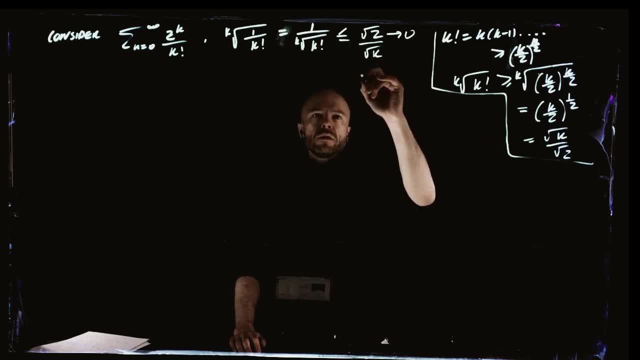 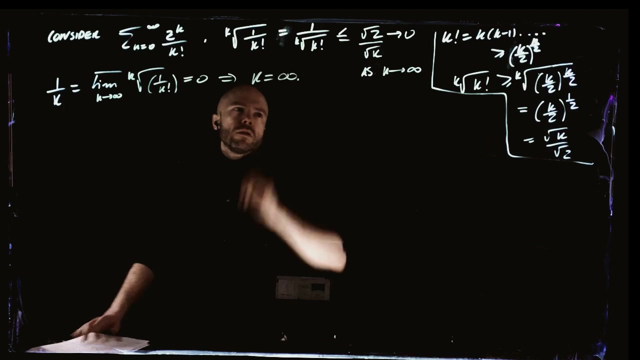 Oops, So we do indeed have that one over. r, which is the limb soup of this thing, which is actually just zero, implies that r is equal to infinity. okay, So the radius of convergence of this thing is everything. It converges everywhere. 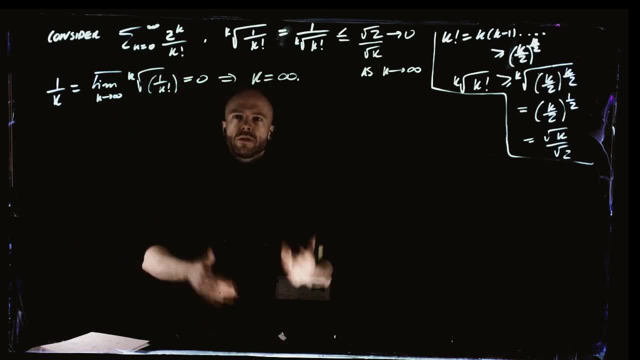 So this thing, this power series, forms a holomorphic function. It's differentiable everywhere And we are going to see what happens if we stick in. just i times theta into this. So notice that if we put in the sum, k equals zero to infinity of. 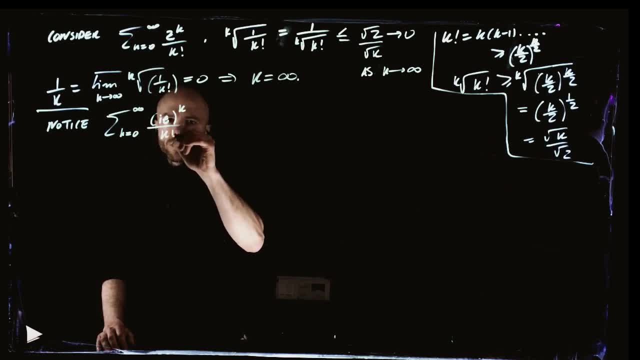 i times theta, the k over k factorial. we can break this into this sum over the odd or the even. The sum k equals zero to infinity. i theta to k plus one Over two k plus one factorial like this, And then the sum over the even. 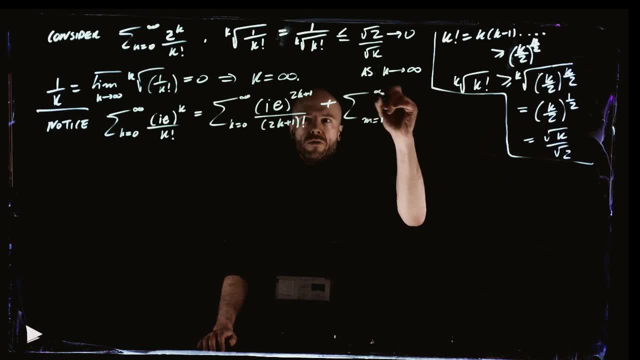 let's say m is equal to one to infinity, i theta to the two m over two m, factorial. And then what happens with this thing? So this is: sum from k equals zero to infinity. Let's pull out this: i to the two k plus one right. 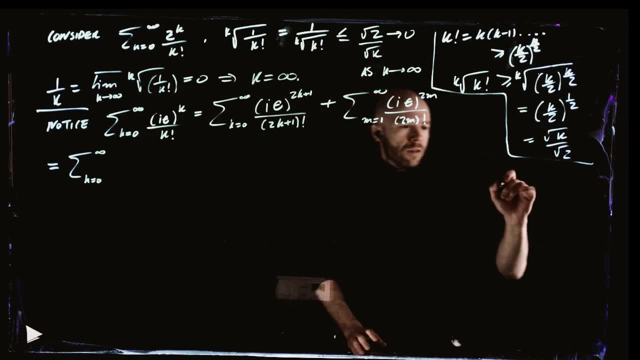 So what is i to the two k plus one? Let's put it over here: So i to the power, two k plus one is equal to i, And then i to the two to the power. k is equal to i and it's minus one to the k. 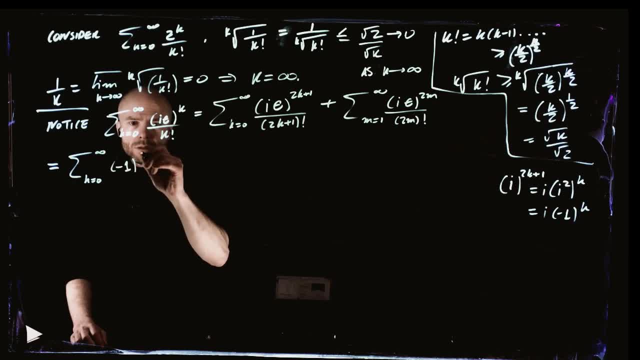 So what we have here is going to be minus one to the k. What else do we have without the i all the way here, and then we're gonna have just theta to the two k plus one over two k plus one factorial. Okay. 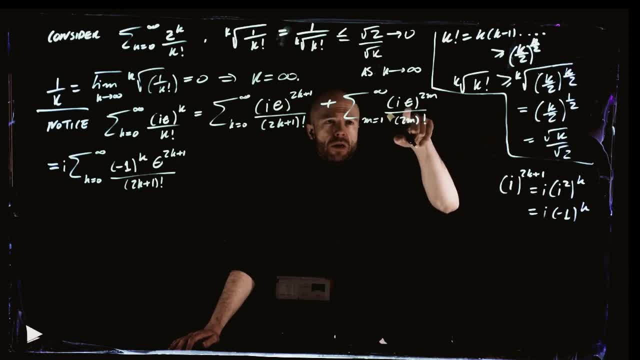 And then from this thing, what happens? We're just gonna have some m equals one infinity and we're gonna have minus one to the m theta, to the two m over two m, factorial, like this And as you guys know, or as you people know, 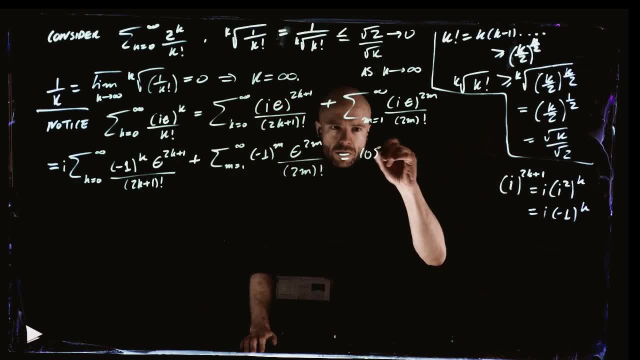 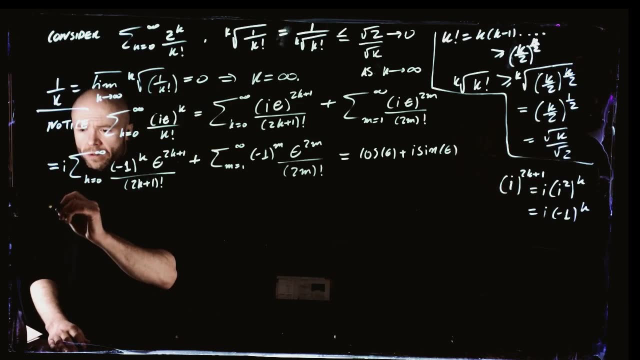 this thing is just gonna be cosine of theta and this thing here is just i sine of theta. So this is what we're going to motivate for the following thing. So we're gonna define the exponential function e to the z, which is e to the x plus i- y, in the following way: 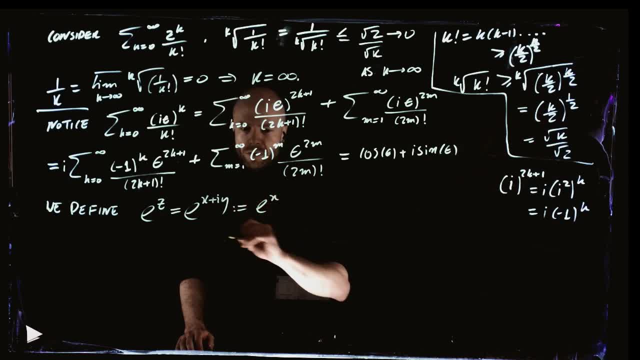 to be just e to the x. so this is the definition: e to the x. we know what it is. it's the exponential function. e to the i theta. we know what it is, it's the phi. ah, okay. 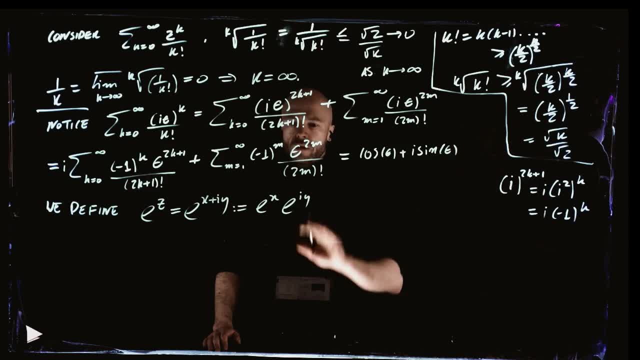 We should perhaps say, we should perhaps write it like this: Write it like this: Cosine of y plus i sine of y. Yeah, So if we define it like this, then what do we know Then? the above calculation is that we have this: 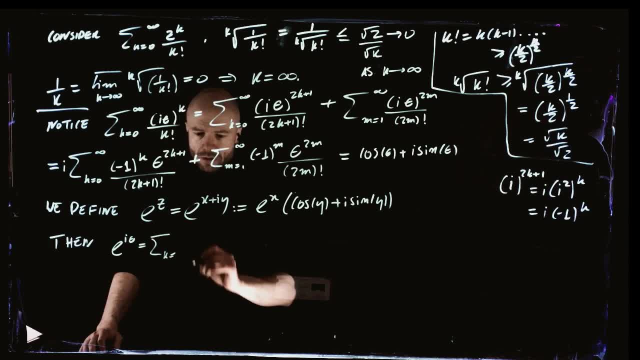 is given by this power series equals zero to infinity. by theta to the k over k, factorial. Yeah, And if we just do this e to the theta itself, or this e to the x, e to the x itself, then just from this thing, 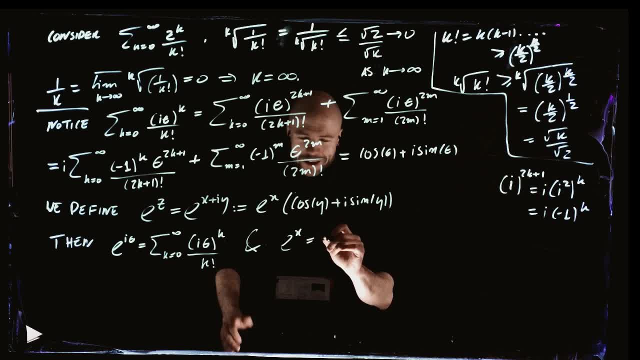 there's no imaginary part. this is just e to the x, So, which is also just given by the power series, the sum k equals zero to infinity, x to the k over k, factorial, as we know from just calculus right. 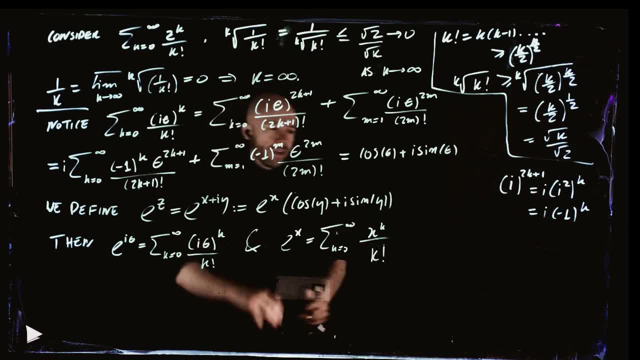 So what we see is that if we define it this way, then it actually agrees with the power series on the imaginary axis And on the real axis, And later we're gonna see that if we define it this way, actually this power series actually represents. 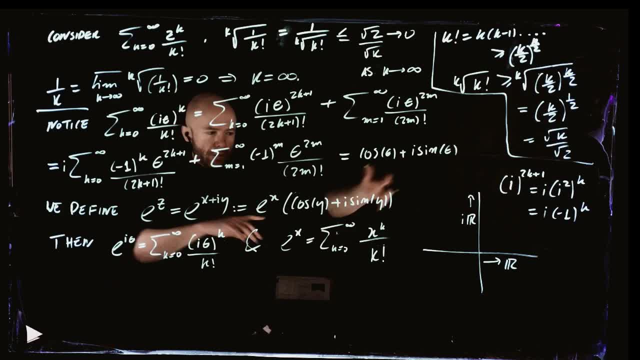 e to the z, everywhere you know. But that we'll have to see later. What you can check pretty easily is that if you define this function like this- and this is a perfectly well-defined function- from the complex numbers, of the complex numbers, 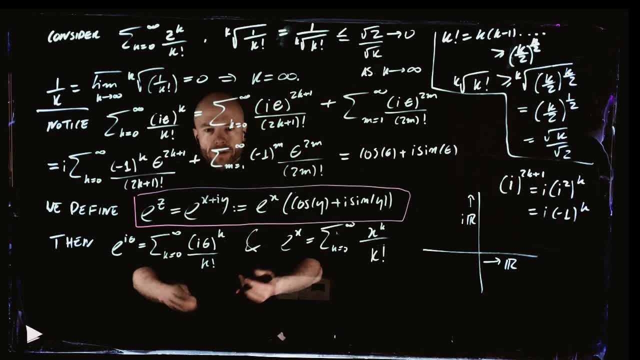 then this thing satisfies the Cauchy-Riemann equations. Just check it, Just do that calculation. However, that doesn't based on what I've shown you. that doesn't imply that it's holomorphic yet, because what I've shown is that if it's holomorphic, 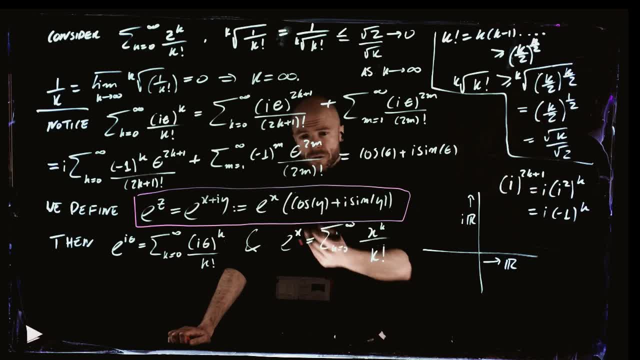 and it satisfies the Cauchy-Riemann. the reverse implication is also true, but that is harder. That can be done with the hypothesis that the function has got continuous derivative fairly easily, but in more generality it's actually harder, Perhaps quite a bit harder. 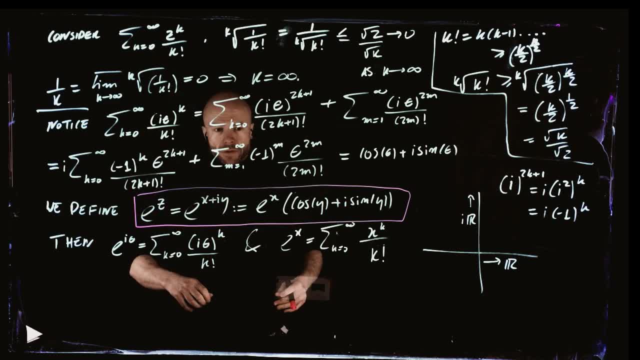 So this thing, okay, is nevertheless, so we're gonna assume this thing, which we can't prove yet, is true. This thing actually is given by this thing, It is given by this power series. So this guy is an example of a holomorphic function. 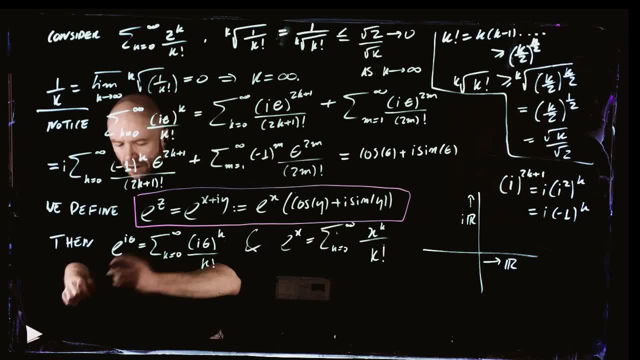 and we're gonna try and understand this, and we're gonna try and understand this, and we're gonna try and understand this, and we're gonna try and understand what it does, and it does surprisingly dramatic things. So see if I can squeeze this in. 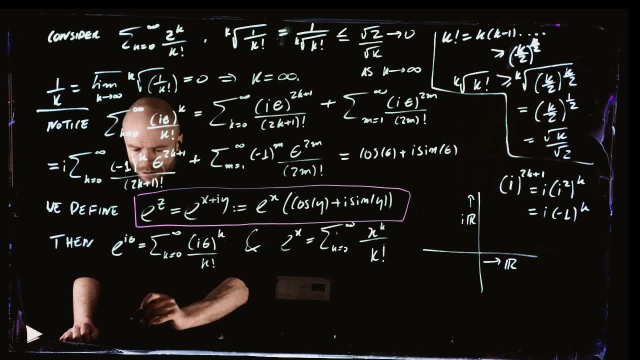 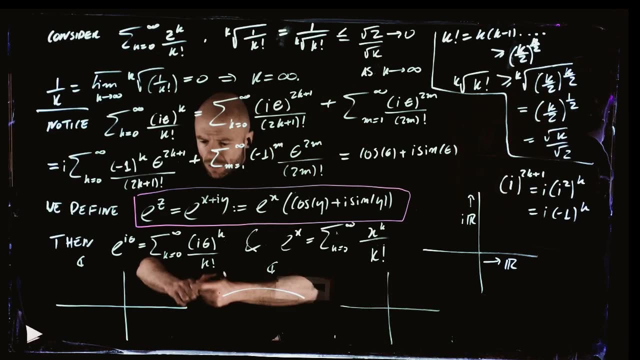 Maybe I can squeeze this in here. So let's take a look at its behavior. Let's look at the complex plane here and let's map it over here with the complex plane. Okay, let's see what this function does If we take a strip. 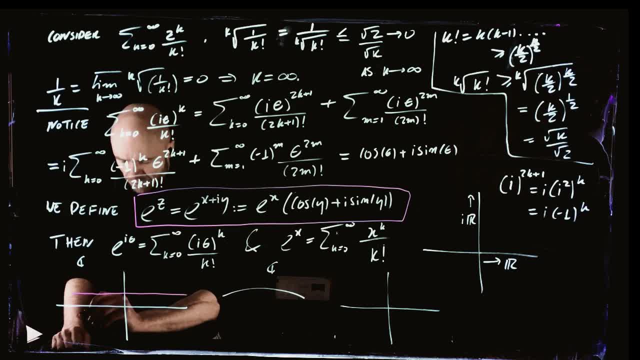 from pi to minus pi and we map it with this guy to the z. let's see what it does. Well, if we take a line like this. so let's fix some x, zero and let's take a line like this: 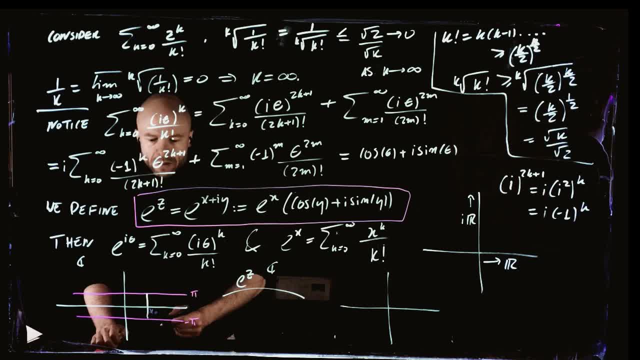 from which goes through this strip. okay, so then we are varying the y from minus pi to pi, but remaining the x fixed right, And then let's look at this definition. So if we do that, then the y is changing. 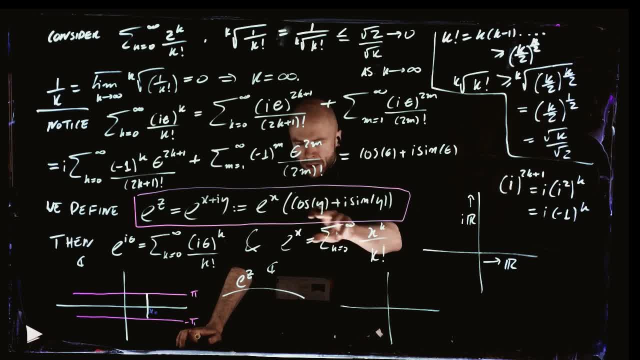 Yeah, the y is changing, yeah, And it's going from minus pi to pi, But the x is remaining fixed, right. So this thing, as we move along this strip right here, x zero is fixed. it's this thing. 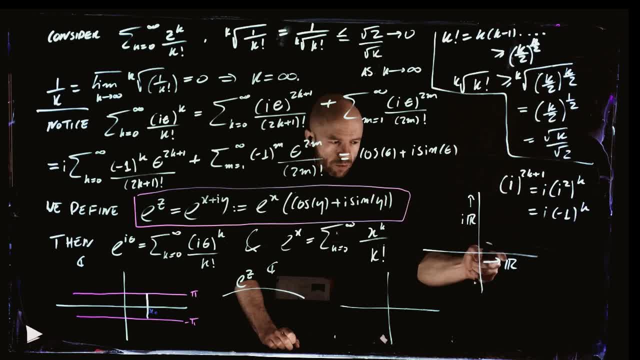 And this thing is just the unit vector in the complex plane rotating around from minus pi, which is over here, all the way to pi. right, That's all that we're doing. So we are gonna get a circle whose radius will be like this: 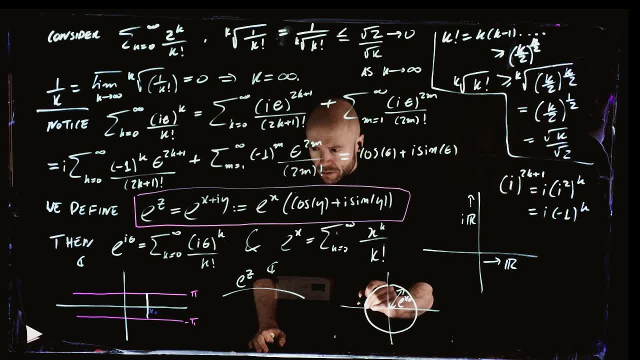 This is the sum of e to the x zero. yeah, As we will start right here, minus pi, and we go round and round and round like this. That's what it does, And if we do the same thing for some x zero over here. 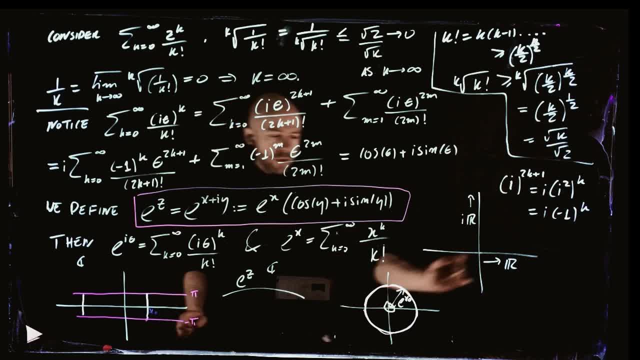 then we get a much smaller circle, And if we do the same thing over here, we get a much bigger circle. So these vertical lines, If we take a horizontal line like this, so now the y is fixed, so it's y0, and we're 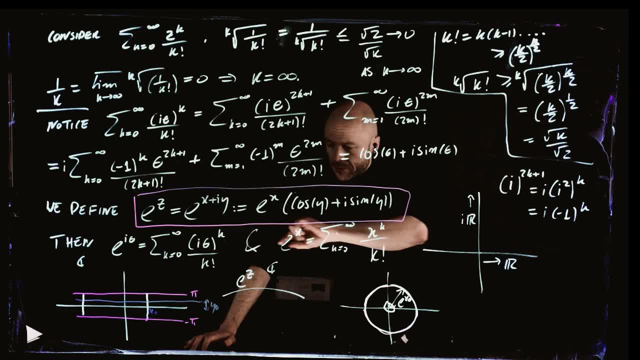 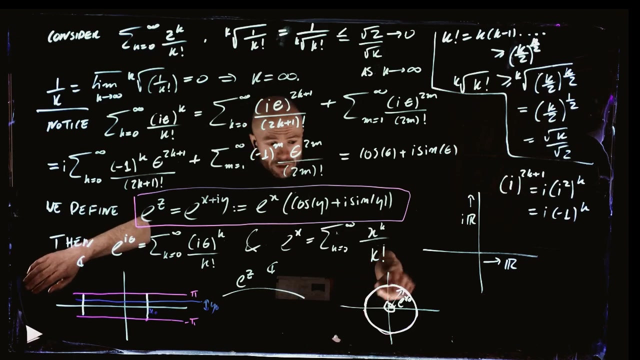 going to have. the x will be changing. then what happens? So y is fixed. so then this is defining the angle. So this is the complex number part, or this is a complex number and this is just a real number. So as x varies, as x goes towards minus infinity, we go towards zero. 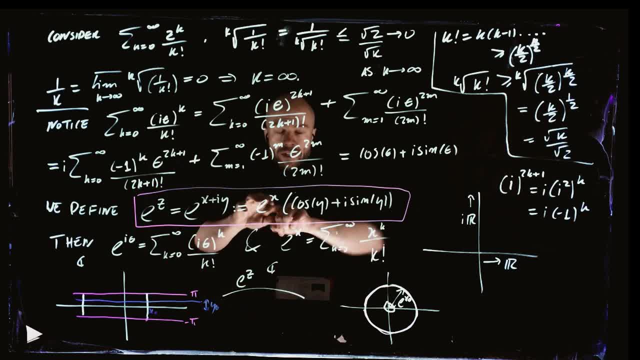 We have e to the minus x, for a very, very negative x, We go towards zero. As x gets positive, towards infinity, we go towards infinity. So then this blue line here is actually going to form the x And this ray is going out like this: where this is where we go towards minus infinity. 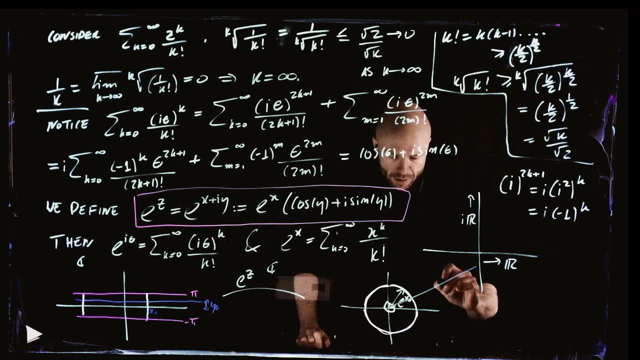 and this is where we go towards positive infinity. And then this thing here is going to be given by angle y0.. And note in particular that at the crossing point of these lines, this point right here, sure enough, they are crossing at 90 degrees. 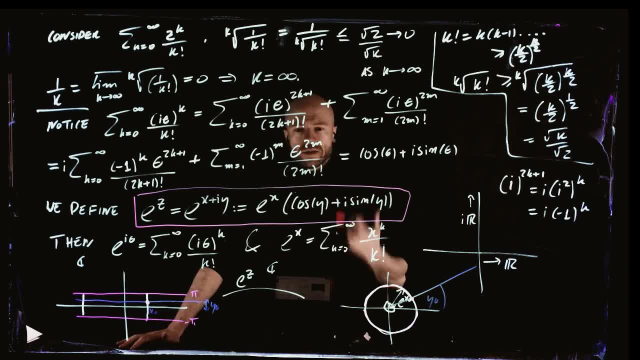 The angle is being preserved, which is what we know has to happen For holomorphic mapping. and what this little calculation also shows is that we are mapping this entire strip onto the complex numbers except zero, right? So we're mapping the entire strip onto the complex numbers except zero. 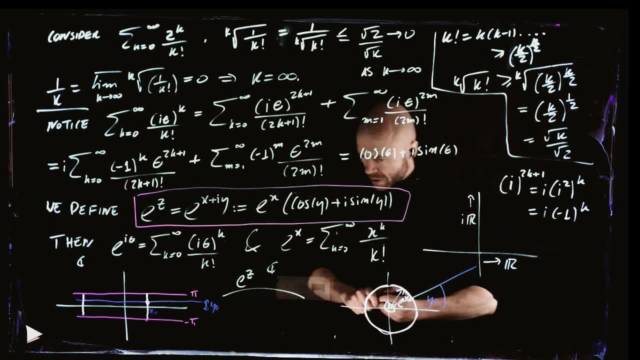 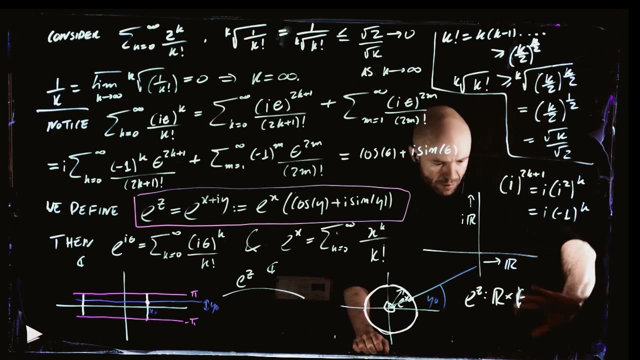 Let's put that here. So e of z sends this strip which you're going to denote like this. so the real numbers cross-product with x. Let's do it like this: i times minus pi, pi. This thing is sent to the entire complex numbers. take away zero, no. 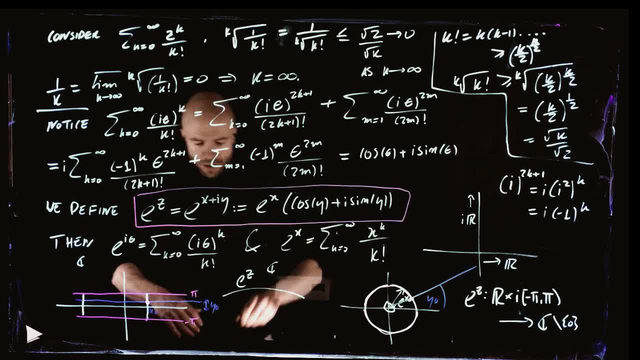 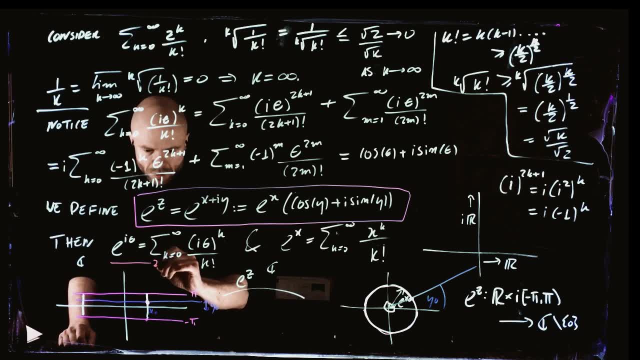 Cool. But from this definition right here, if we consider the strip which we just get from moving up a little bit from pi to 3pi, Okay, then the same thing is going to happen, right, Because this expression here is periodic in pi, right? 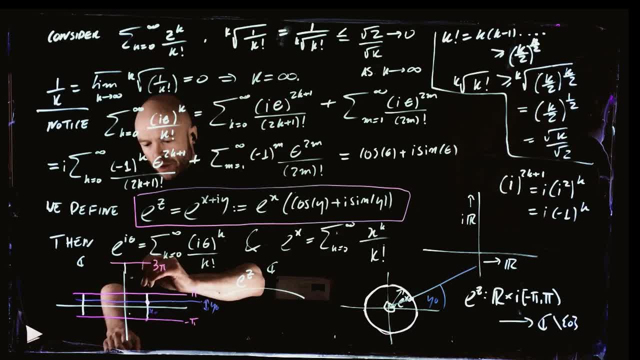 So, whatever is happening here, we move up by 2pi from here. exactly the same thing is happening. right? So it's going to map this strip to the same thing. right, So we have. we can cut up the entire complex plane into these horizontal strips of width. 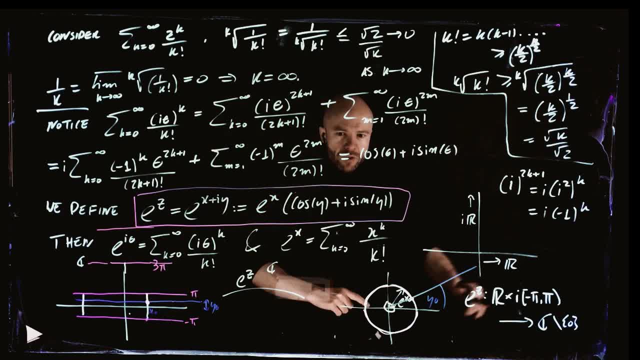 2pi, And every single one of them is wrapped around the complex plane right in the image. no, So this is a really crazy behavior. This is much more strange and complicated than z to any power k which we can sort of. 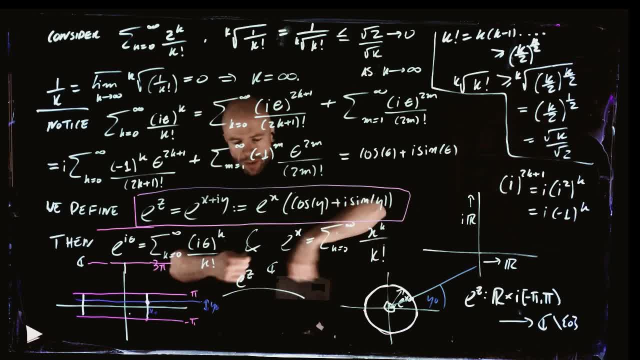 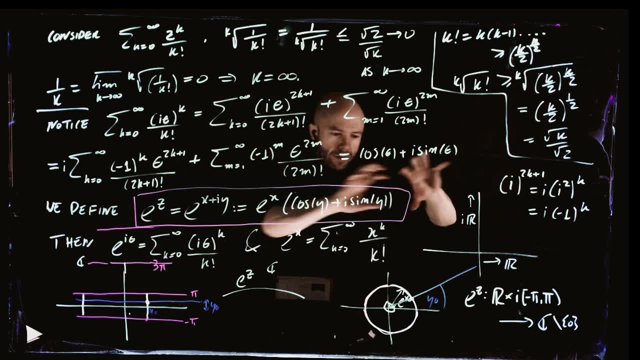 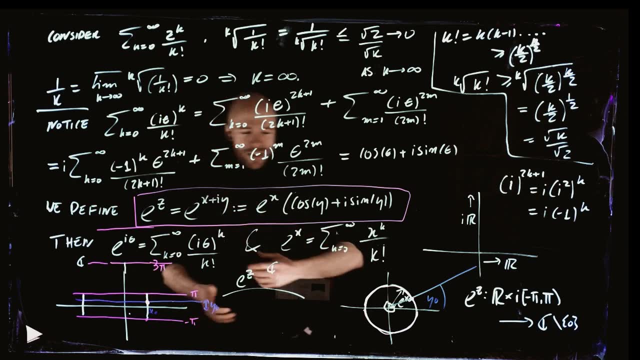 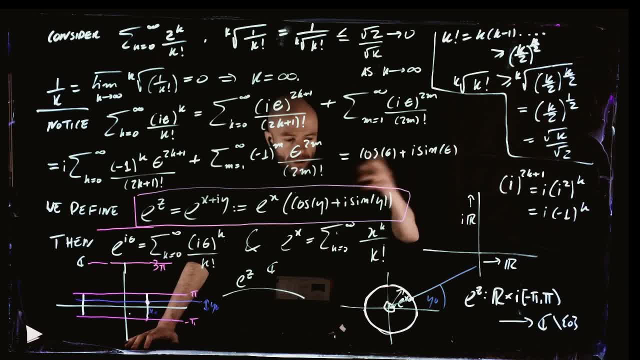 point, And later we'll see- it's even more than differentiable. it's differentiable to any order, In fact it has a Taylor series, it's analytic, you know. So very dramatic, strange behavior for a function that locally preserves angles everywhere. 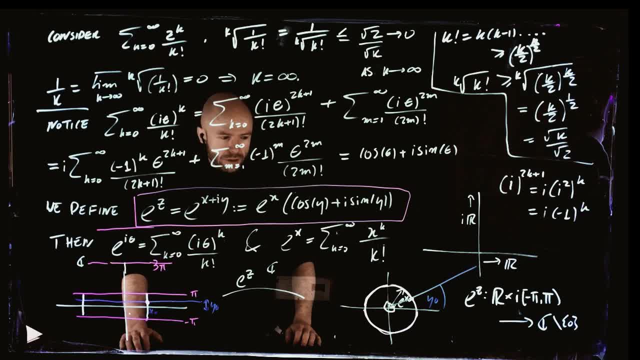 and is differentiable everywhere. It's quite a surprise that such a thing exists, Um, but it does, and it's not, it's not. these things are not particularly hard to work out. so We have this particular example, uh, of a strange complex, of an unusual, surprising. 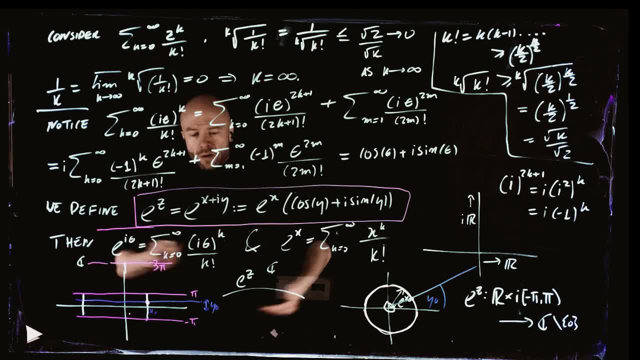 holomorphic function And note it also recovers the the ordinary exponential function that we know. because if we just look on the real line, then then on the real line, then this is: this is the exponential function. Right, If y is just zero, it's just the ordinary exponential function. 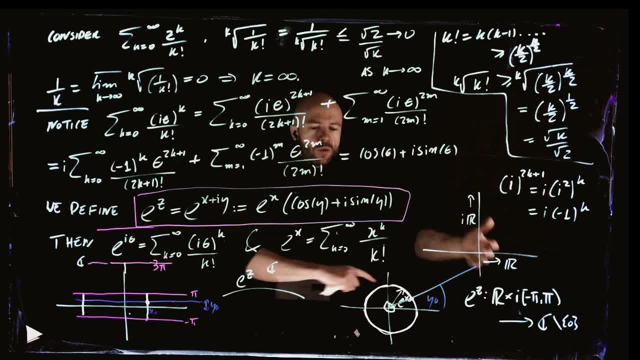 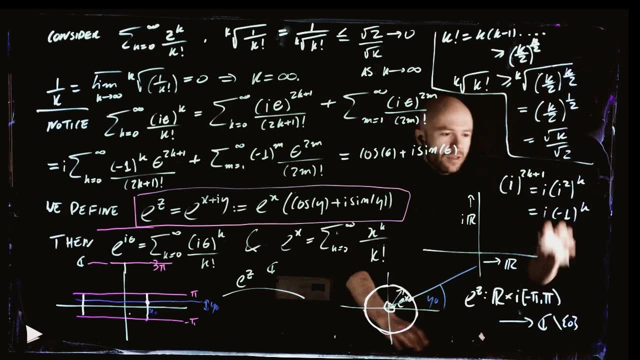 So this monster contains the guy that we know well from calculus, and it just contains it. when we restrict what happens to the real, the real numbers, It sends the real numbers to the real numbers you know. So part of the familiar old exponential function we've known about for a long time, uh is 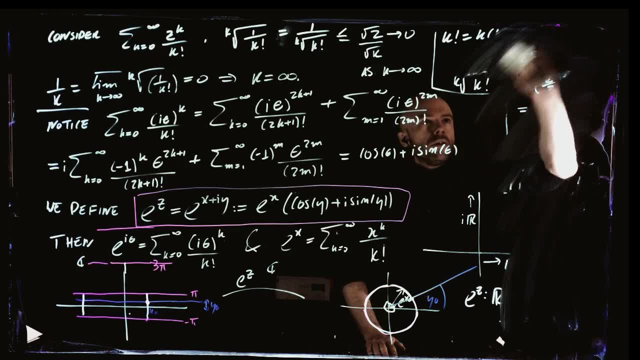 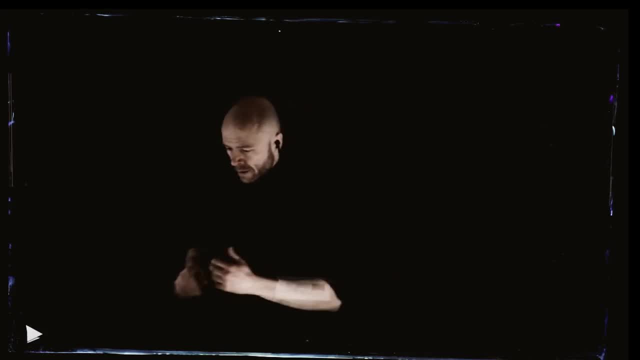 inside this guy. All right, we're gonna talk about log functions And and trick functions when I erase this board. Okay, so let's discuss more this strange function, what it does. So we've seen that it takes all these horizontal strips like this: uh, this is minus pi pi. 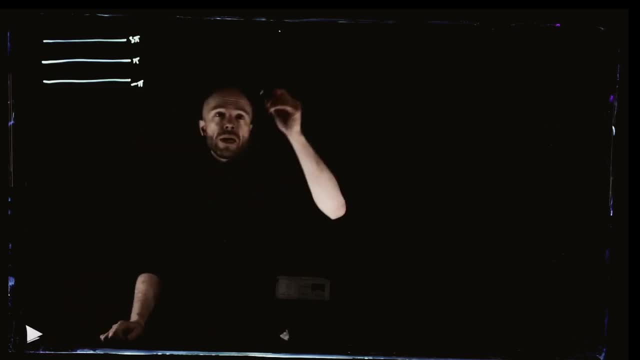 three pi and so on, and it maps them, wraps them all around the complex numbers at zero, Yeah, Okay, So, in particular. so this is: uh z goes to e, to the z. If we take some complex number here, say w, and we ask ourselves what gets mapped onto. 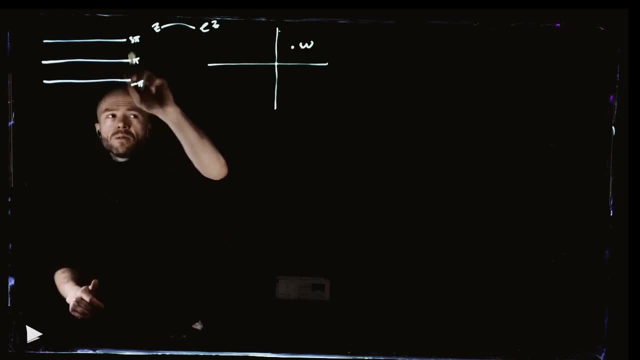 w. well, as we've seen for any one of these strips. for short it maps around the entire complex plane except zero. So in each one of these strips we're gonna hit this at least, in fact, we're gonna hit. 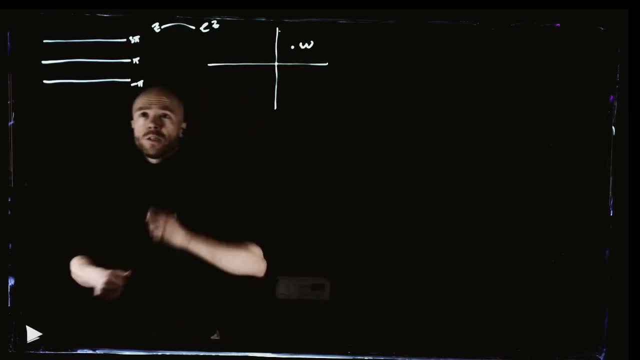 exactly one time, kind of clear from our construction, One of the strips. there'll be one guy that hits this right And because whatever's happening in the strip is happening on every strip moved two pi up, two pi down for any multiple of two pi actually, then the same thing is gonna happen here. 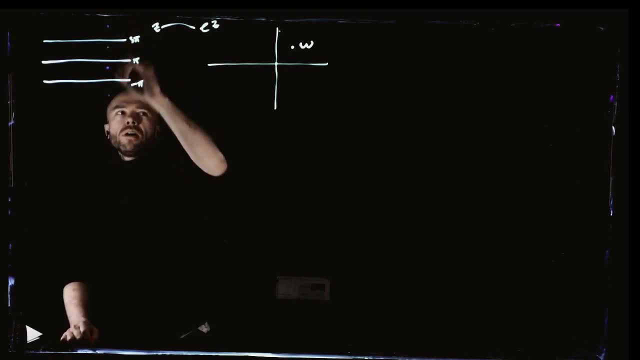 and then here, and then here. So all of these blue dots, we mapped all onto w. so so the inverse of e to the z is no longer gonna be a one-to-one function, which you know it is on, you know one-to-one. 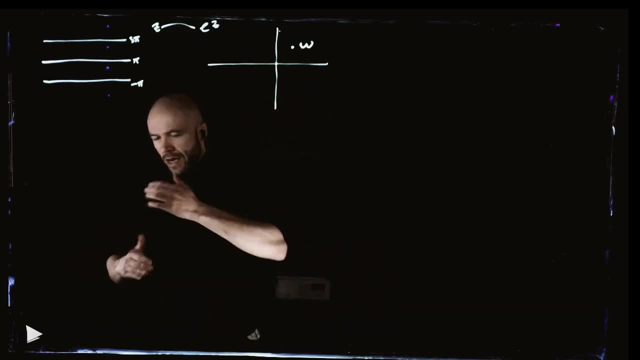 The real line when we do calculus e to the x is a monotone function satisfies the horizontal line test. It's invertible. We have a. the inverse is called natural log. No such thing happening here, right, But the the inverse seems to have quite a regular structure. 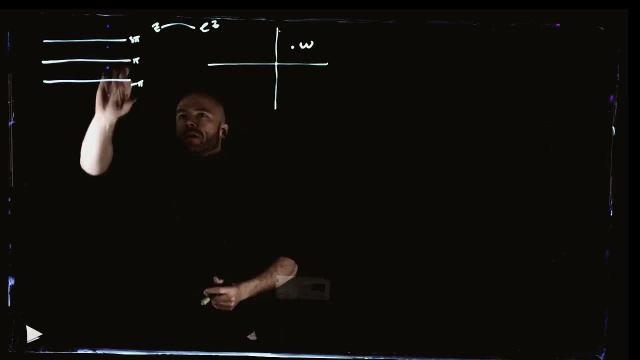 In fact, if we restrict down to some particular interval from minus pi to pi, then then it will be invertible, right, And there's only one copy. There's only one copy happening there. So we call some notation. so, given z inside the complex plane, then we can write z as: 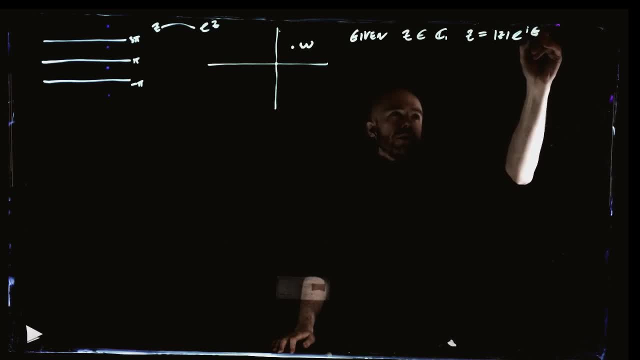 mod z and then e to the i of theta, for some theta right, And theta is not unique, because every multiple of two pi is also gonna do this representation, But we can choose what we call the principal argument, which we're gonna write like this: 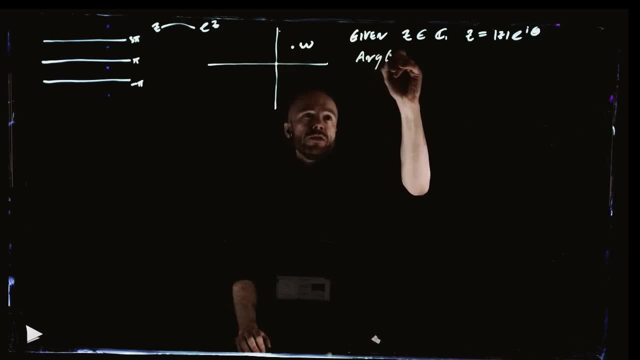 so arg of z is the one particular number which, like this, which satisfies this, which is inside this interval. There's only one guy which will satisfy this, so that z is equal to mod z, e to the i arg of z, right. 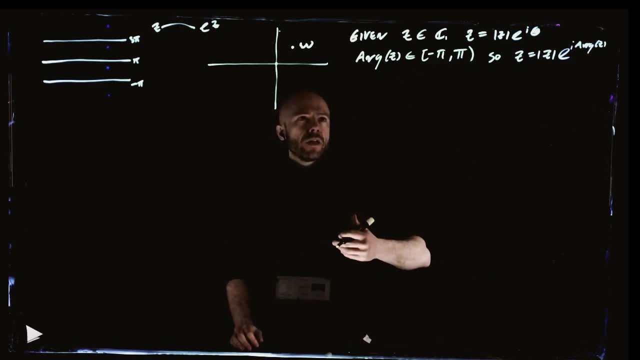 That's the one representation of the angle inside this, Inside this particular interval, And this thing we're gonna define to be equal to arg of z plus two pi, k or or k, which are integers. So this thing is actually an entire infinite set of complex numbers. uh, sorry, sorry. 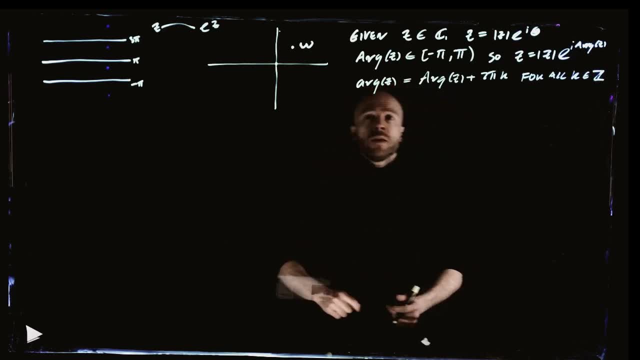 this is an entire infinite set of numbers of angles, right? So Okay. So this is- uh, this is at least notation in Zill's complex analysis book. I, I guess somewhat standard notation. So let's try and understand what the inverse of e to the z will be. uh, given that we have 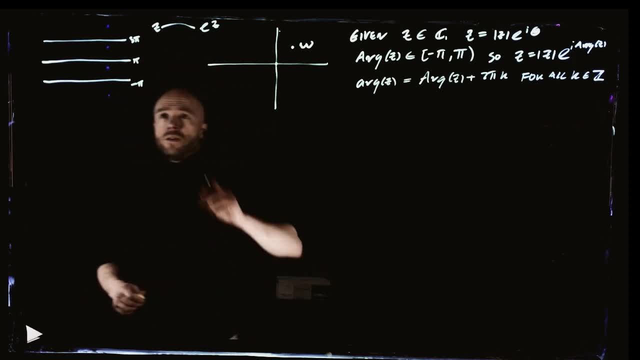 a fairly good picture of the way it behaves. Uh, so if we restrict to just minus pi to pi, then what happens? So if let's say, let's call it, we'll give it a name, let's call it: log of z minus pi. 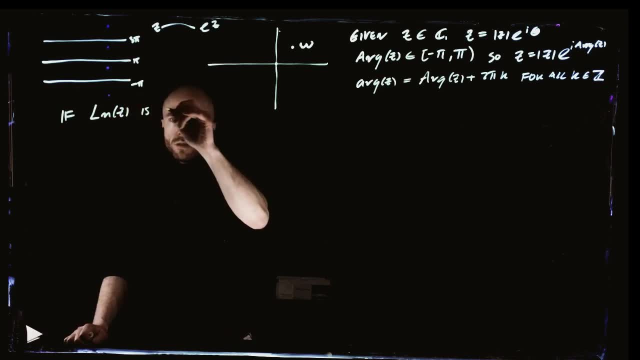 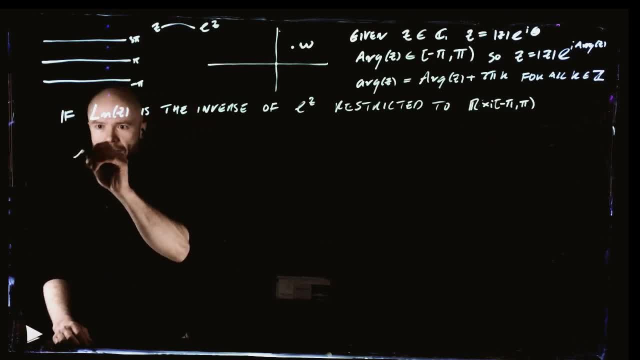 Okay, Okay, Okay, Then what? uh, what properties will it have? Then it has to have this property that e, Oh, it's right, like this, z has to be itself again, right, but then this thing is just given by e times the real. 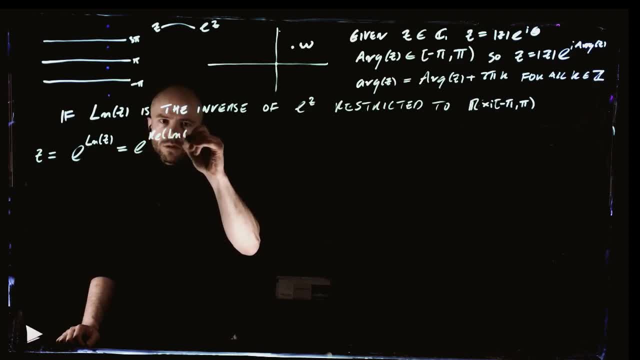 part of this guy. Okay, plus, i times the imaginary part of this guy which, by definition of e, how we've defined it, is this thing: e of the real part of log of z, and then times e to the i, the imaginary part of log of z. 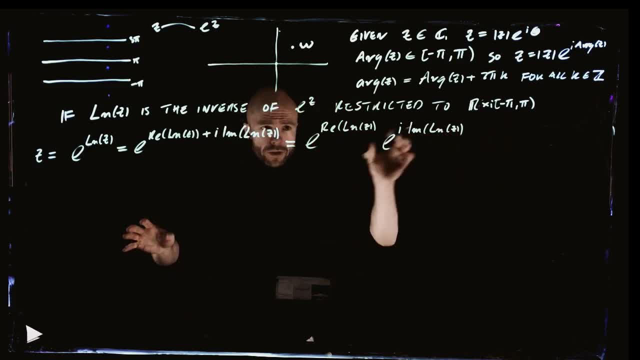 So if we just take the absolute value, this thing is just a complex number of length, one right. So taking the absolute value, we have that mod z is equal to just e times the real part of log of z And therefore, if we take natural log now, 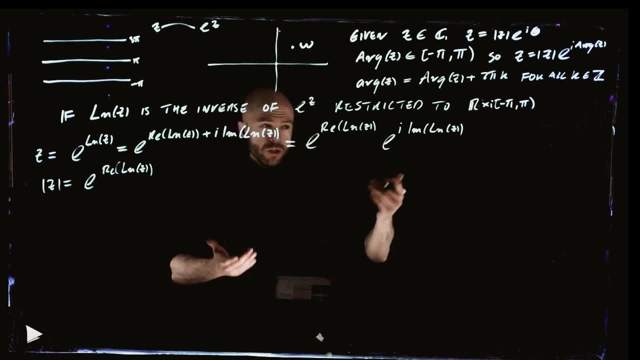 I mean real natural log, natural log from the real numbers to real numbers, which will denote by log to the base e. So let's put over here: log to the base e. is this natural log from real numbers to real numbers? If we do that, then what happens? 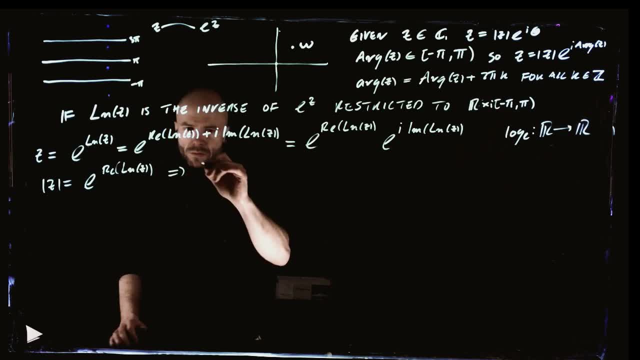 Then we have that log to the base e again, this is notation from Zill- is equal to this real part of log of z. So we understand what the real part of this function has to be right Just by taking absolute values. 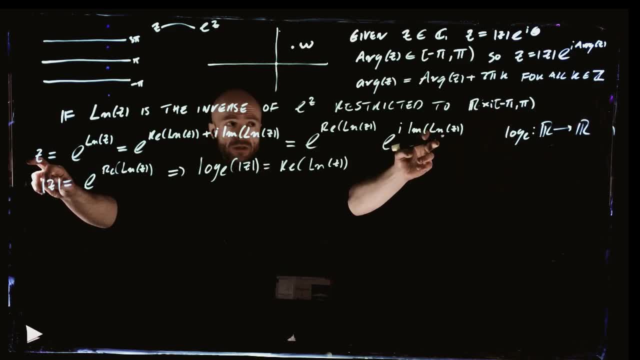 And now, if we look at the direction of these complex numbers, right, Just in this guy, then the direction is denoted by this thing, right? So we also have that z is equal to mod z, e to the i times log of z. 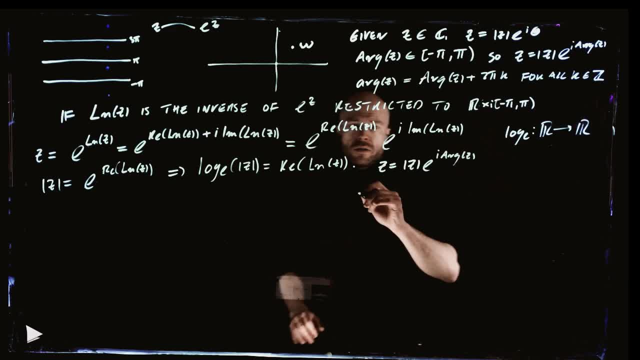 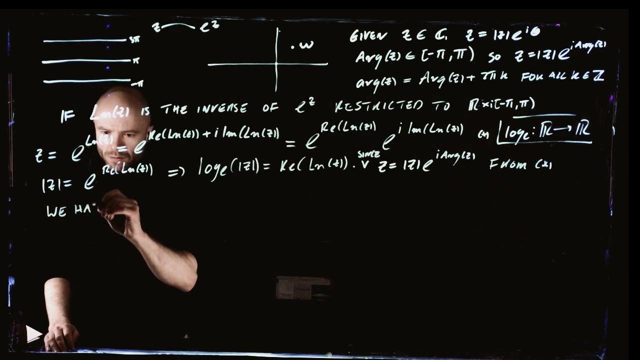 which is equal to this thing, right? So let's put this since. so, from the line above, let's call this thing star from star. we have, we have what, Um, we have that, we want to have that here. 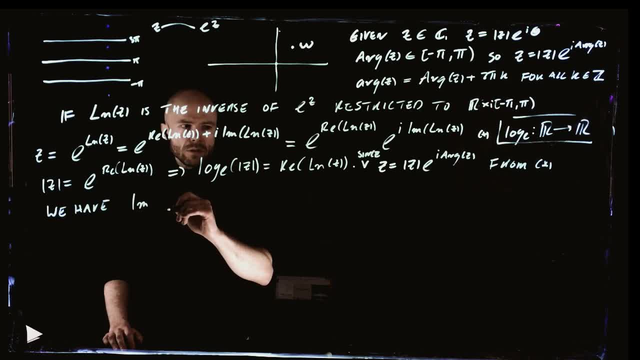 of z has to be equal to this thing plus any 2 pi k right. So we have from star and the fact we've just found out that mod z has to be this thing. we have that e to the i times the imaginary part of this thing has to be equal to e to. 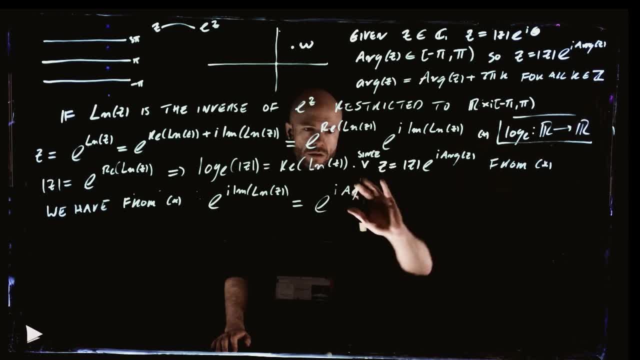 the i arg z. Yep, and the only way that's true. we could also write e to the little i arg of z. This implies that the imaginary part of log of z is equal to arg of z plus 2 pi k. Let's write it like this: ie, that's the same as little arg of z. 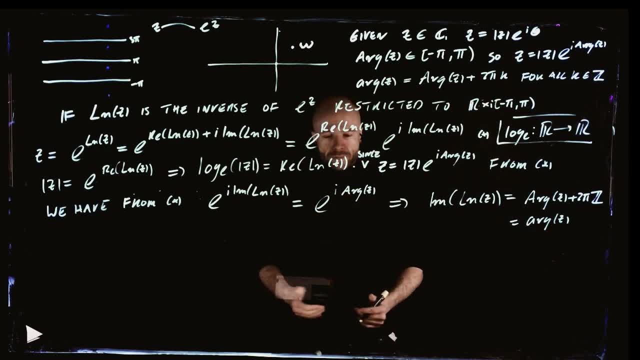 Yeah, So what that means? it means we've completely defined what log of z has to be right, Because its real part over here is given by this. so it's log the base e of mod z. That's what it does to the real part, right? 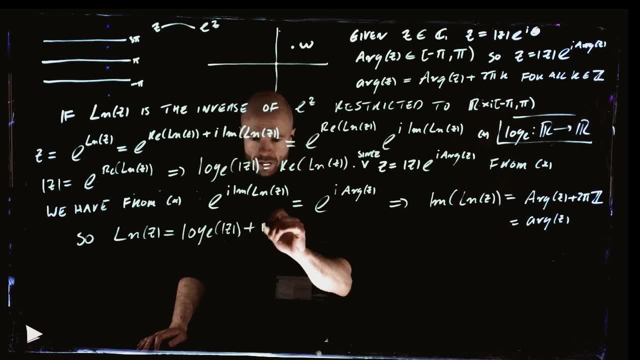 And the imaginary part we've got from over there is this which, as we know, is like this infinite set. It's a set of real numbers. right, Arg of z? is this infinite set of real numbers? Did I erase it already? 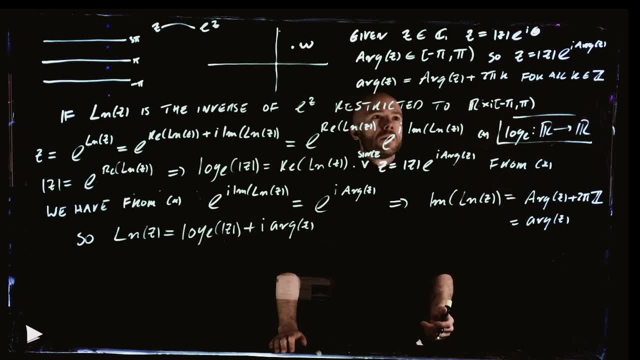 No, here it is right. Yeah, and let's compare it to a picture. Well, if we restrict this thing just to minus pi over pi, then it is indeed a well-defined function and we would have this thing. Yeah. 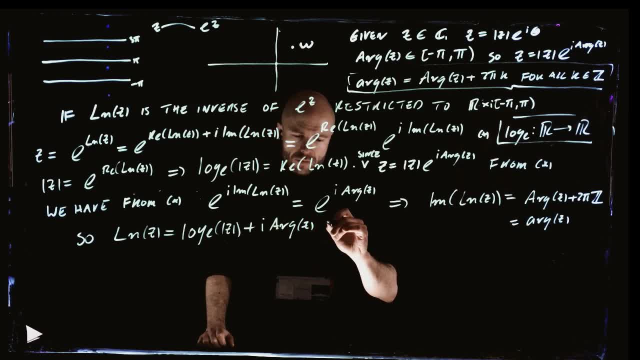 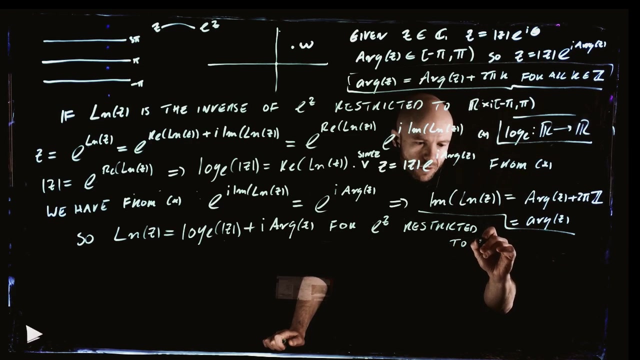 Yeah, Yeah, That's not true really. Or e to the z, restricted to just one of these strips. Does it have a three to four? No, it doesn't. So then if I restrict this part over here and then put it one over here, 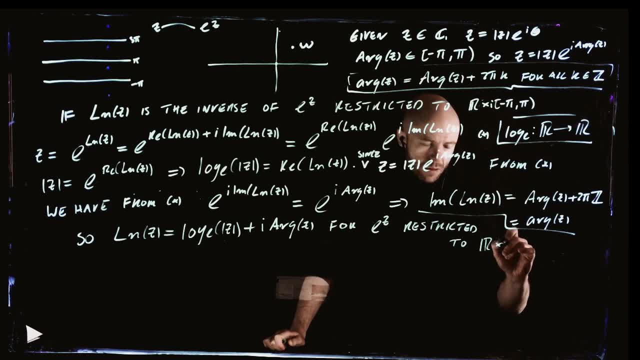 umm a zero. Yeah, It should Shimla ome more product. because in this case, if we were restricting z to one of the strips or the inverse is going directly back to the strip, then it is not arg plus anything else, it's just capital arg. 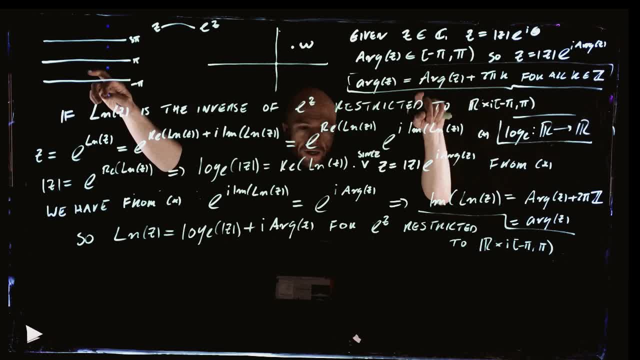 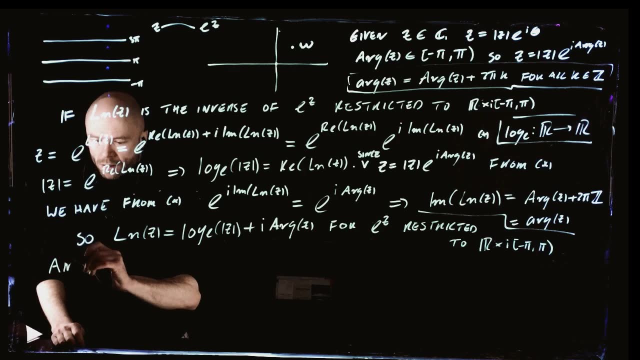 by itself, which is by definition just in this strip. So the restricted mapping from here to the entire complex numbers minus zero is invertible by this guy. yeah, and the more general inverse is not a traditional function, it's not a one-to-one or many-to-one function, it's a one-to-many. 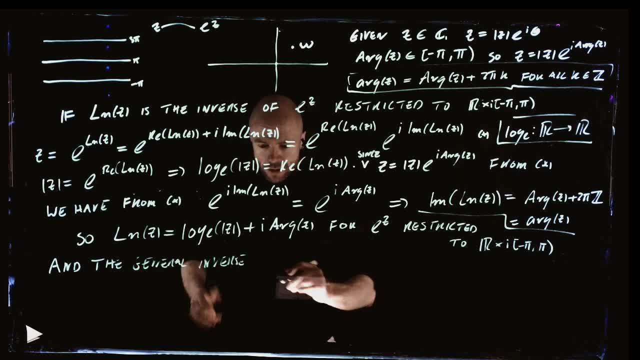 function. it's a set-valued function. General inverse is given by this. So better perhaps to have different notations for these two guys. maybe I will, I don't know. I will say log n and then put a tilde or something: log e, z, and now we have this. 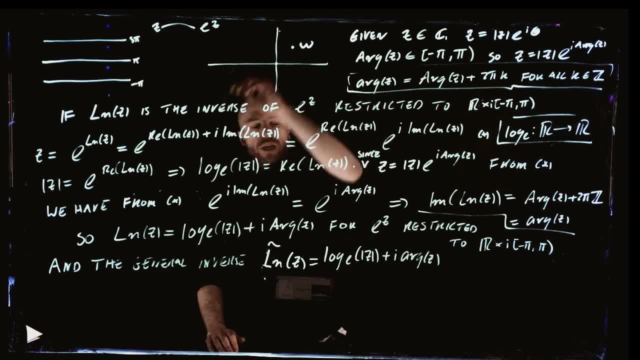 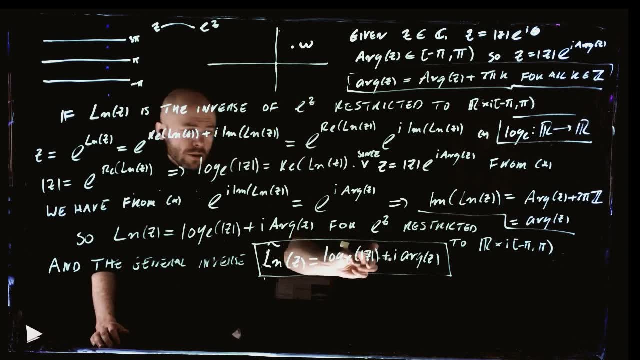 So it's every z over. here we have the entire infinite set. this is defining an infinite set right, and that infinite set has its real. it's every. every number inside that infinite set has its real. its real part is given by this, but the imaginary part changes and it's 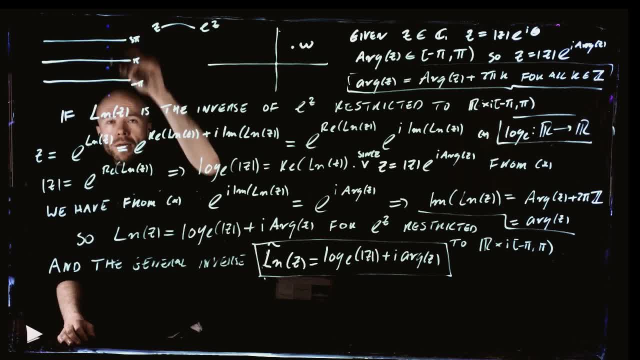 exactly this picture here. it's exactly all of these dots right here. right, because each guy has just moved up or down two pi i from the other. yeah, so we recover in the language of maths what our picture tells us. Our picture tells us that that's what happens if we consider all the images, all the z that 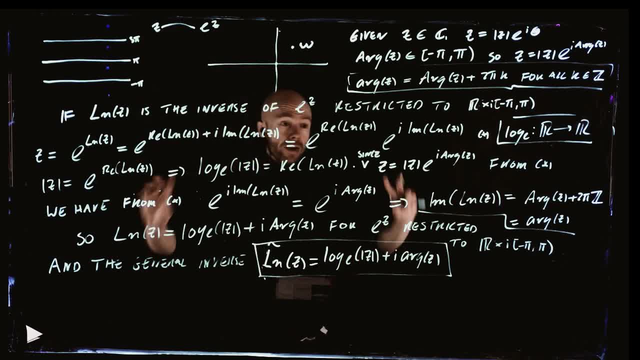 map onto w. we get a thing like this, and then the language of math confirms it. that's actually what we get. So that is the log, the general log function, and again it's a more complicated, complicated type guy and interestingly, this is, this is, I mean, this is a very classical subject, this 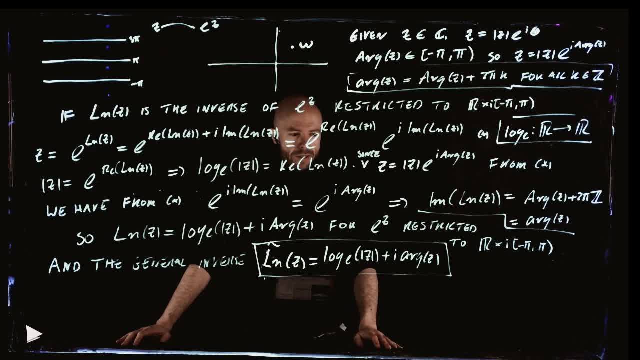 is 17th and 18th century math and this is one of the origins of of of the theory of Riemann surfaces. so I don't know how much you people have studied a little bit about this, but but you presumably heard of these things called manifolds. which are these, these sets in which 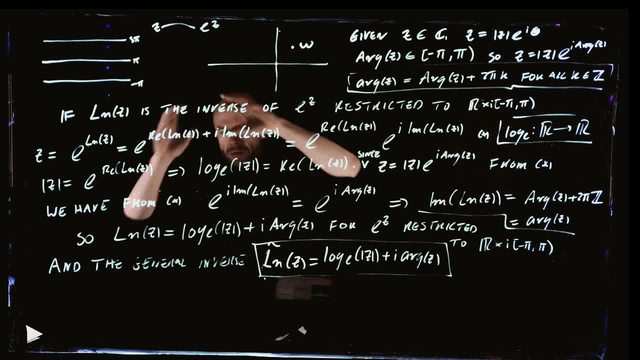 are more general than arbitrary, just portions of space. they are sets that we define with, with a diffeomorphism from open space- Yes, Okay, subset of Euclidean space to some part of the set and there's different ephemophysisms that cover the entire set and they act in a nice way across each other, right? 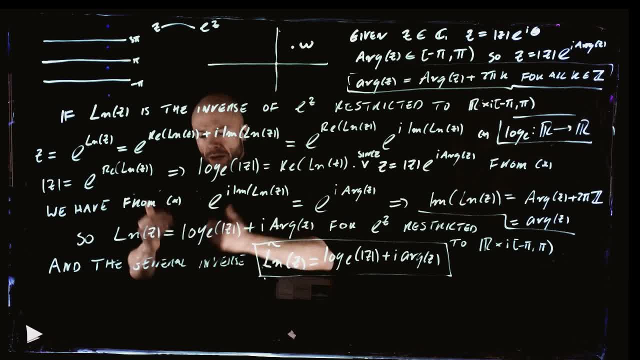 So locally you can describe it as being something like Euclidean space, but not globally right, And this was initially kind of a concept that was somewhat difficult, took a while to develop. One of the reasons for developing it was to try and understand things like this, because 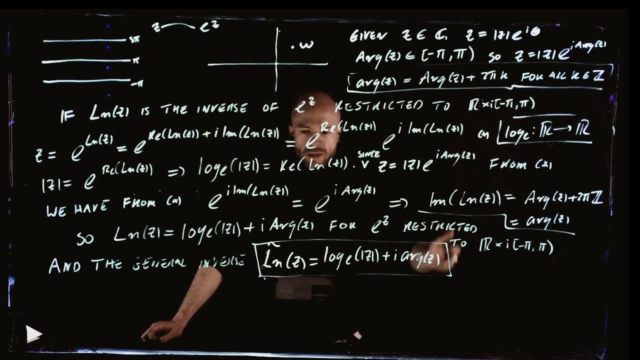 if we don't want to think about this as a function which is mapping one-to-many, if we want to try and understand this as a function that is actually one-to-one, then we can't map it back into the complex plane. We have to map it into something called a Riemann surface. 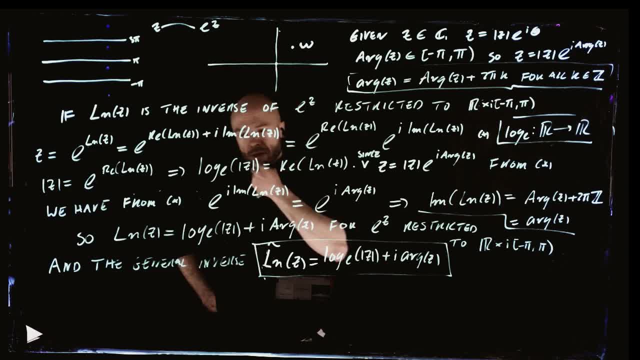 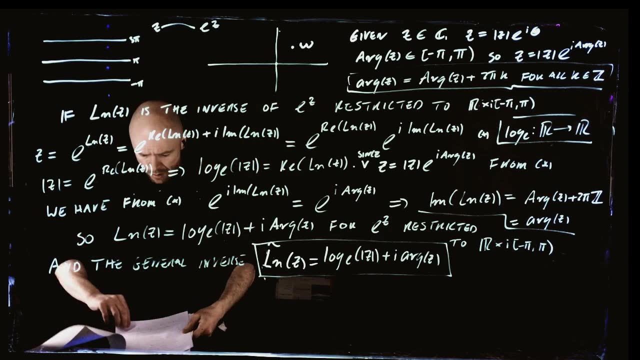 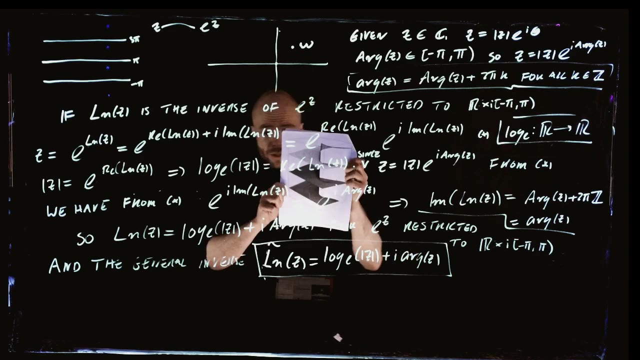 Which is It's just a complex manifold. It's a manifold where the charts are made up from analytic mappings from subsets of a complex plane onto that particular set, And I downloaded a picture from the internet like this, so this thing here would be something. 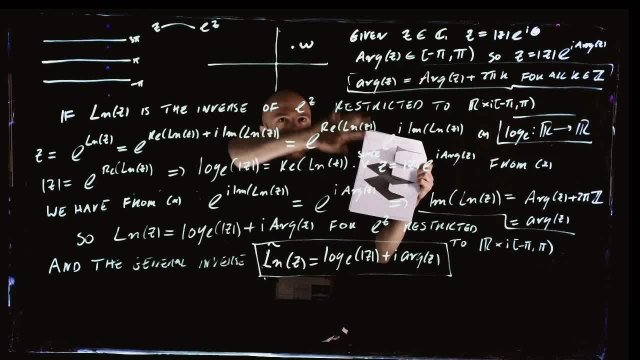 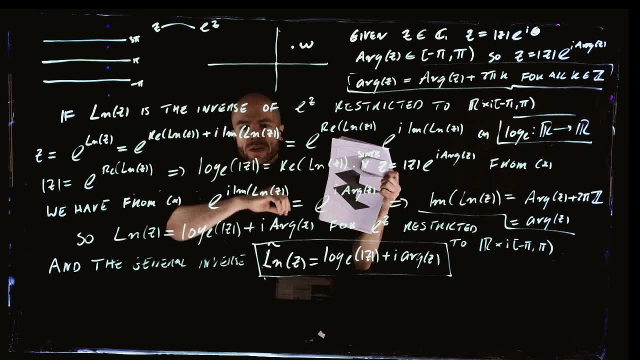 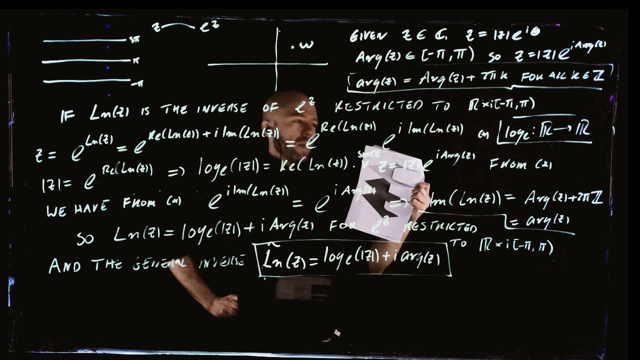 that would allow us to map With log from the complex plane onto a guy like this, where we wouldn't have the issue of having multiple, multiple values, Because this thing would, This thing would make sense. So this is a little bit off topic, but nevertheless. 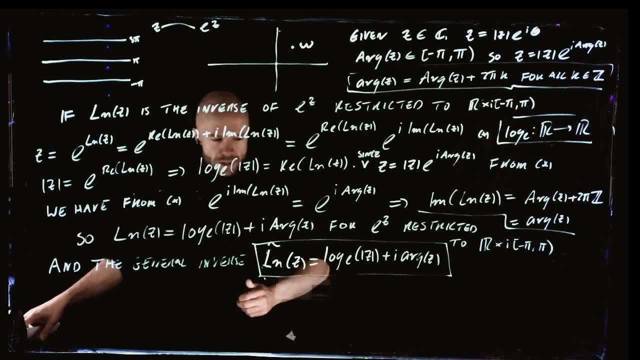 This, historically, is Is, Is, Is, Is, Is Is initiated the development of a lot of math. We had to stop thinking about just dealing with subsets of Euclidean space or subsets of the complex plane, but we had to define this more general object where we do analysis, where we do calculus. 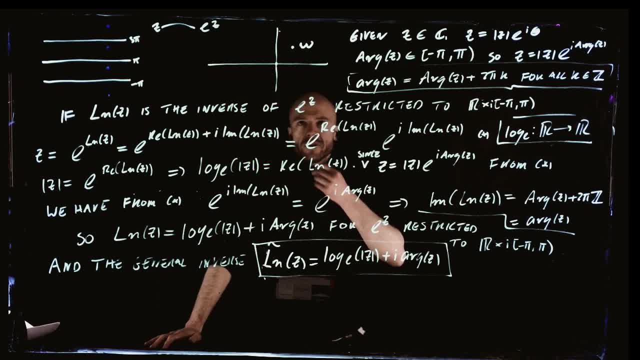 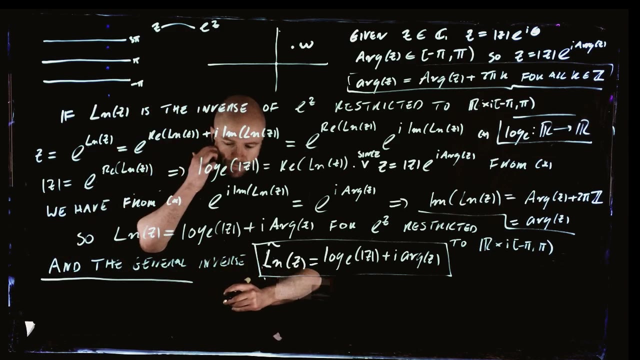 called the manifold in order to make sense of things like this. Okay, All right, so that is the general expression for exponentials. Let's try and develop complex trig functions from this. so let's do the following: So what do we know? We know that e to the i theta. 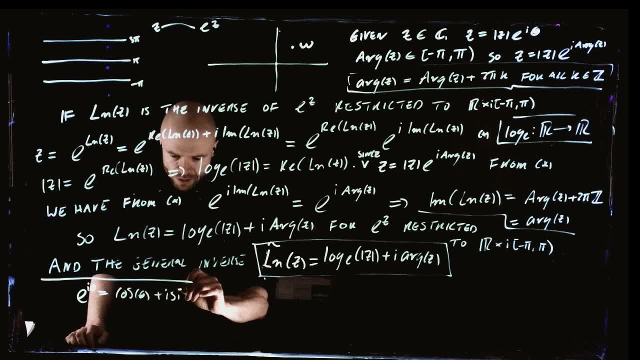 cosine of theta, sine of theta. so e to the minus i, theta is cosine of theta minus i, because sine is odd right. So we put the minus theta through, we pull it out This. So if we add these together, things together. 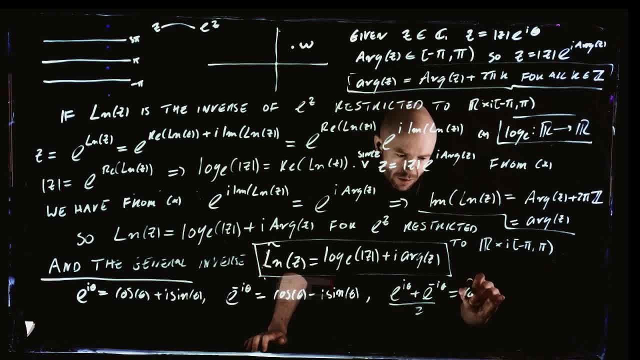 and we divide by 2, we just get cosine Yeah, And a similar calculation. If we take e to the i theta and now we subtract e to the minus i theta, right Now the cosines are going to cancel and we divide by two, i we're going to get sine of theta. 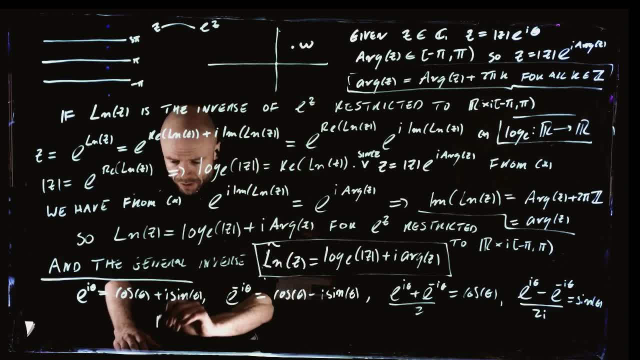 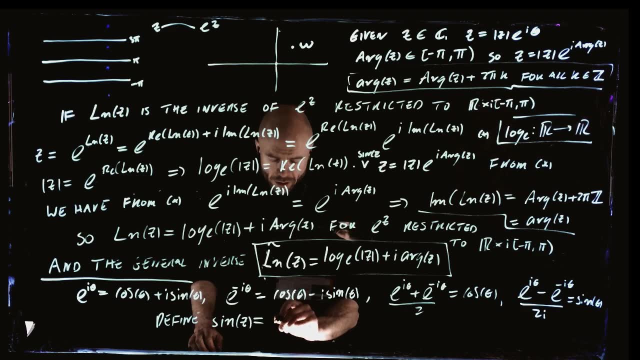 And that's going to allow us to define these functions like this: From the complex plane to the complex plane, we're going to find sine of z from this thing to be e to the z, sorry, i of z minus e to the minus i of z over two i. 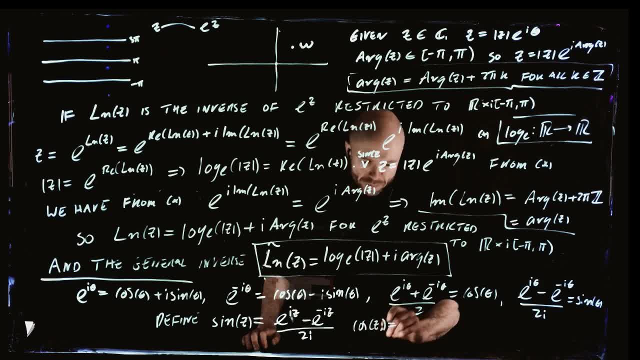 and cosine of z to be e to the i times z plus e to the minus, i times z over two. And since e to the z and therefore e to the i, z and e to the minus, i z are perfectly well defined holomorphic functions. we're just subtracting two. 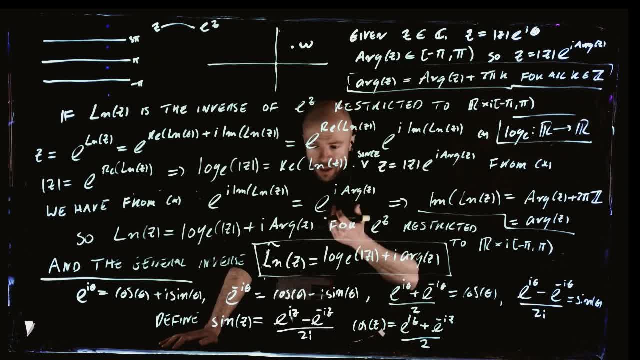 dividing by a number, multiplying by a number. So this thing is a holomorphic mapping as well. just because what we know about holomorphic mappings? we can add them, subtract them, multiply them, multiply by a constant. all that stuff, And this guy too. 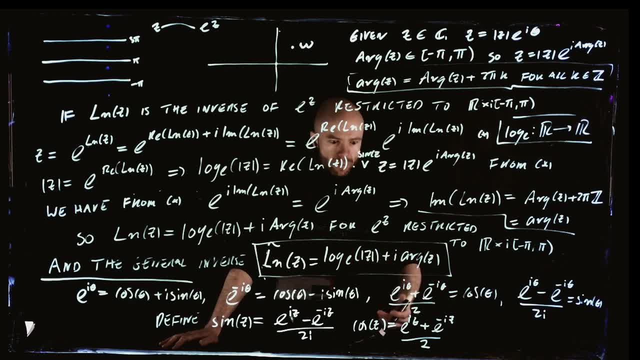 So this thing, these things are perfectly good. holomorphic mappings: they're defined everywhere, differentiable everywhere, And if we restrict down to just theta being between minus pi and pi, then these guys give us back. well, in fact, if we just restrict theta, 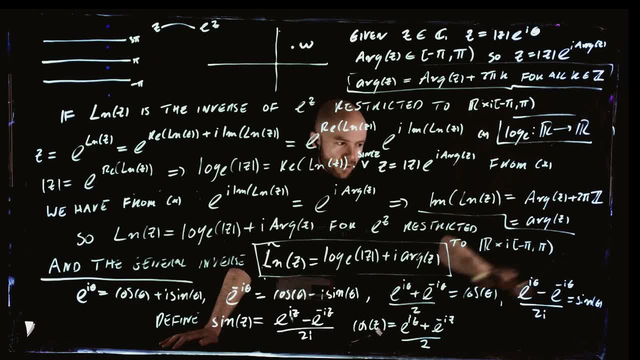 to be on the real line. these guys give us back ordinary sine and cosine. So these things are different. These are deformations of the complex plane, preserving angles, right. So we have the complex plane over here. it's mapped to the complex plane over here, right? 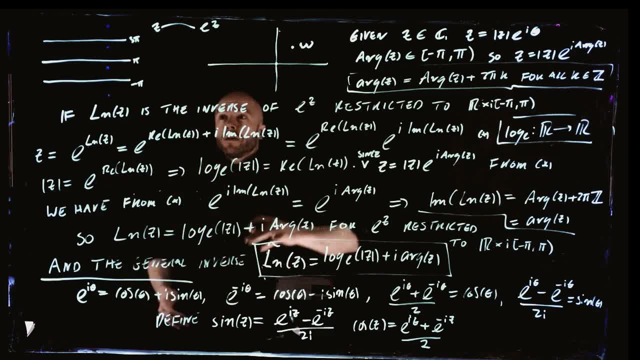 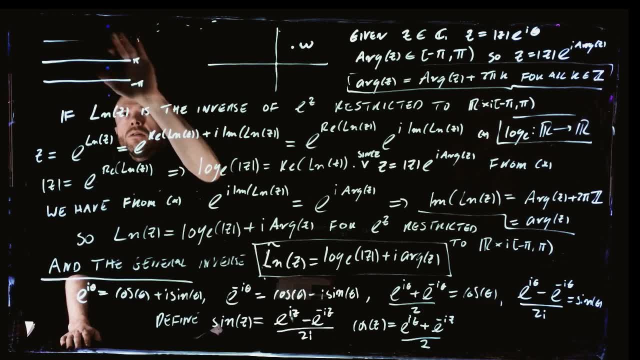 And if we just look at- just put this picture here- if we just look at what's happening on the real line, then we recover our ordinary trig function. So if we think about this thing, z goes to theta, z goes to sine of z. 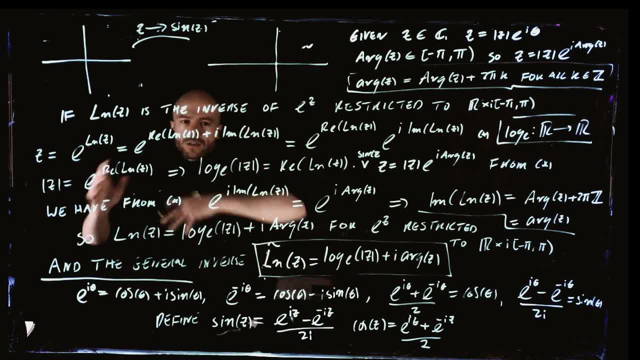 And this is deforming the complex plane. you know It's deforming it in a locally angle preserving way. But if we just take a line like this- see what's happening here- then it is actually just mapped to minus one to one. 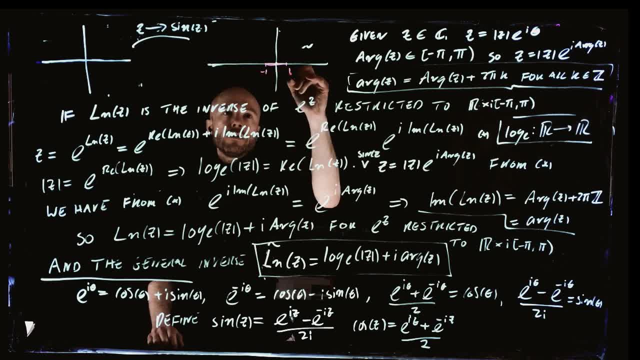 Like this: the real line is mapped up to here, okay, And the behavior of this guy on just the real lines is just our sine function, right? So what this means is that these common trigonomic functions that you're familiar with for many, many years now. 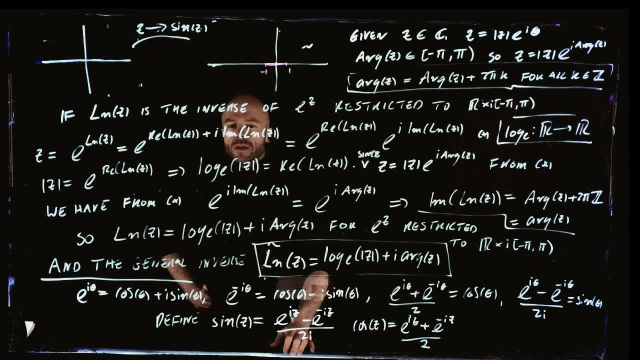 you learn in middle school, I guess, and indeed mathematicians were familiar with for a long, long time before the discovery of complex analysis. they are just a part of another function, a more general function, which is actually acting in a nice way. 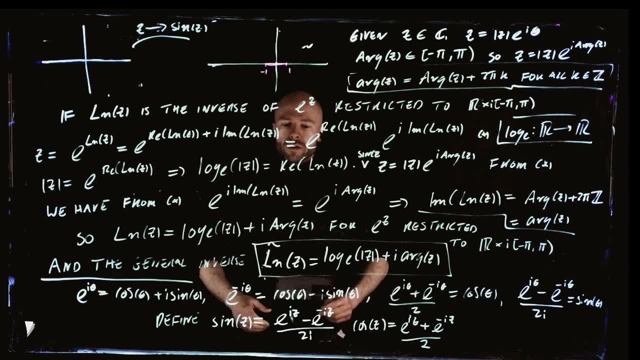 in a completely nice way from the complex plane to the complex plane. So all this stuff of studying trigonometry, all this stuff that you learned, you're just studying the behavior of this guy on the real line. you know, You're just studying the behavior of a little bit. 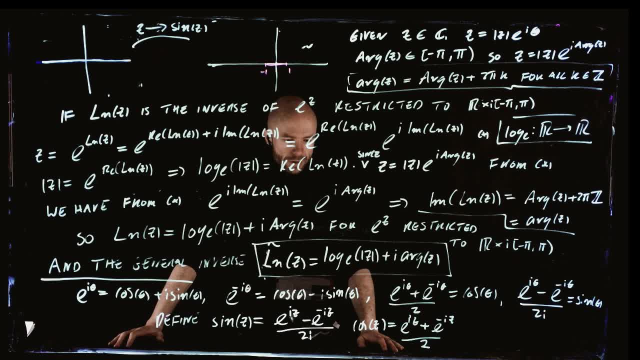 of this more general function. It is just a slice through these particular guys. it's just, I don't feel like saying, like a shadow of some bigger thing, and that must have come as quite a surprise to the early mathematicians who discovered this. because you would think, 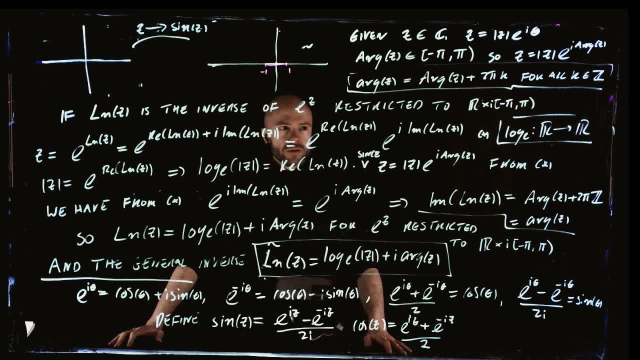 you'd know everything about what sine and cosine. they seem fairly simple things, But no, all along you were just looking at just a piece of something much bigger, much more general. And this guy, it's holomorphic. but as you can guess, 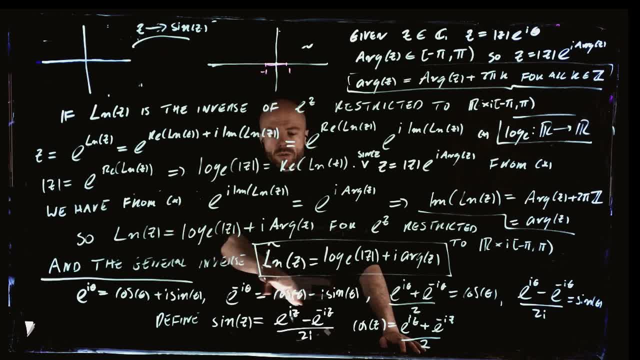 given how wildly non-one-to-one this is, this guy is too. this guy is also wrapping the complex plane many, many times around in the image, And so it's actually a kind of a kind of a. it's kind of a quite a interesting guy. 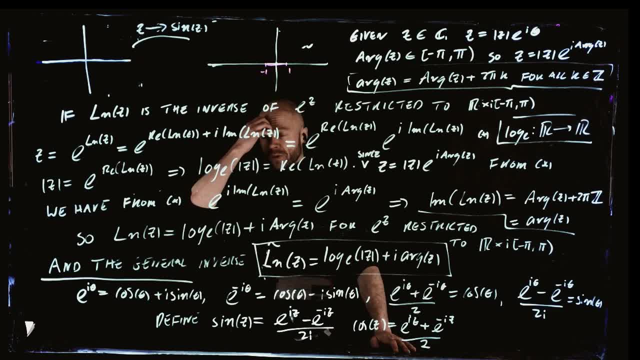 It's quite a complicated- not complicated, but quite a rich- has quite rich structure this holomorphic function. It is richer and more complicated than you might think And it's kind of like a little bit of a taste of what happens more and more in higher math. 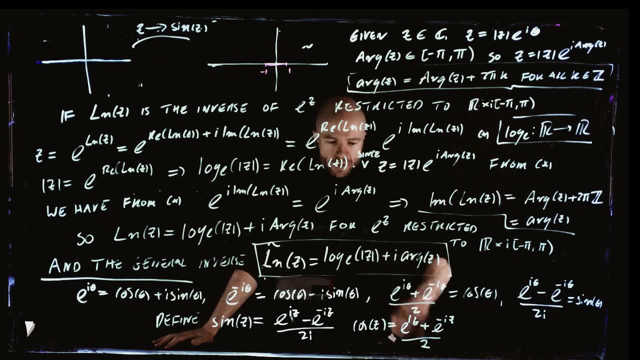 that you think you understand something. you think it's some mathematical object that's been studied for a long time and many properties about it, And within within that era, you can prove these properties with this collection of techniques And then later it's discovered that that thing 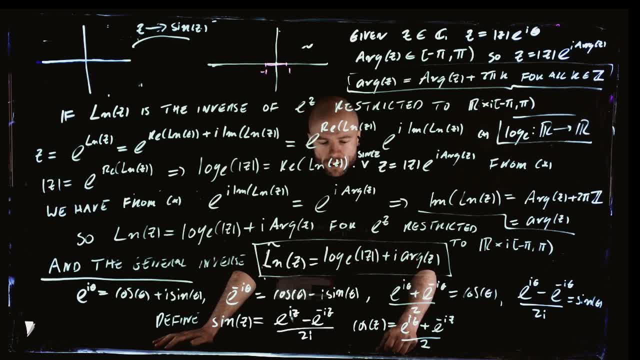 is just a special case of some other object, and the other object is way more rich and has a lot more structure than the thing that you were studying and all the stuff that you know is just a special case and all the stuff that you know is just a special case. 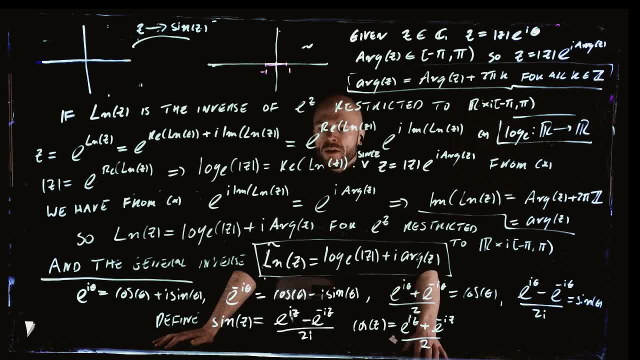 and all the stuff that you know is just a special case, special case of stuff about the more general thing and you were just looking at a slice of the real story, just a. you just had like a, like a. you were just looking at a like. 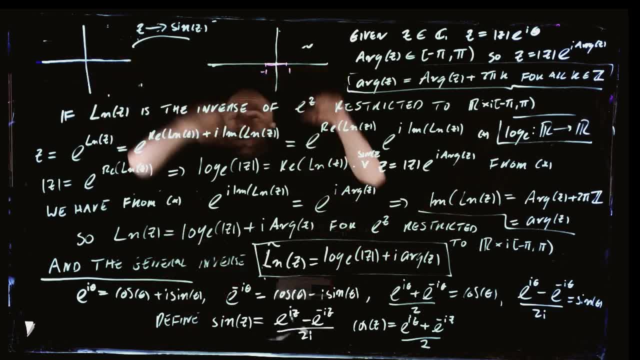 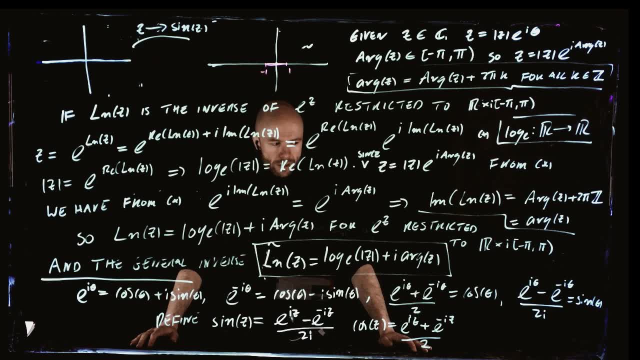 a tiny kind of like. this is just literally a slice of the of the action here. So it's it's kind of cute the way that this- you can see this already in this- in this field that is common, easily understood, well understood things- trick functions are part.